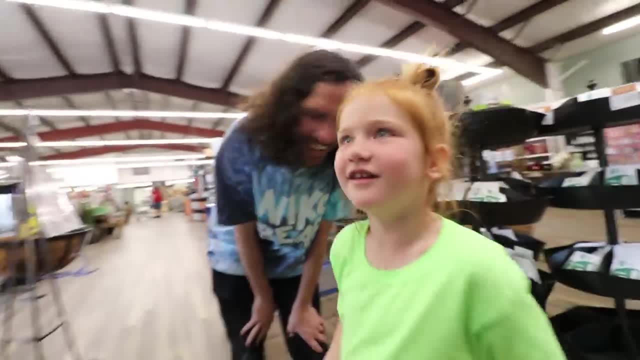 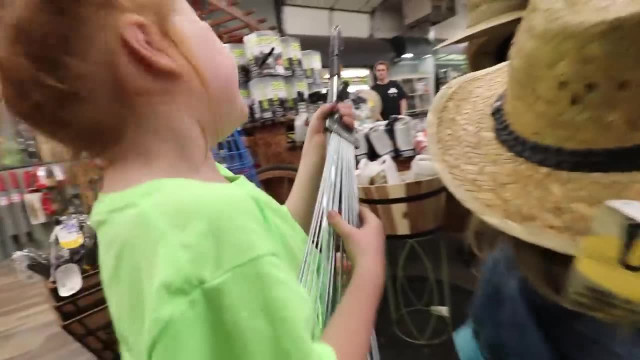 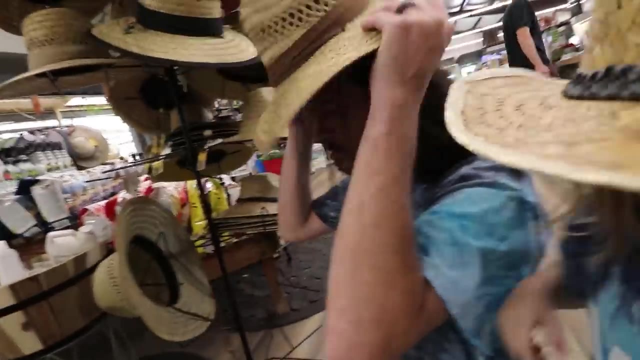 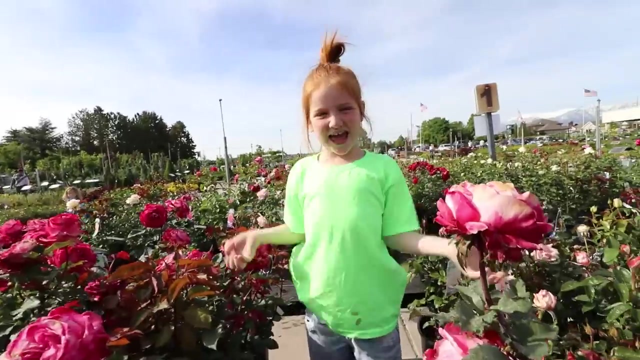 Does Shark Dog like Brussels sprouts? Yeah, he loves them, but they make him fart Pretty cool. Welcome to A for Adley. Yeah, Got some garden huts, Boo, Scary town. Welcome to A for Adley. 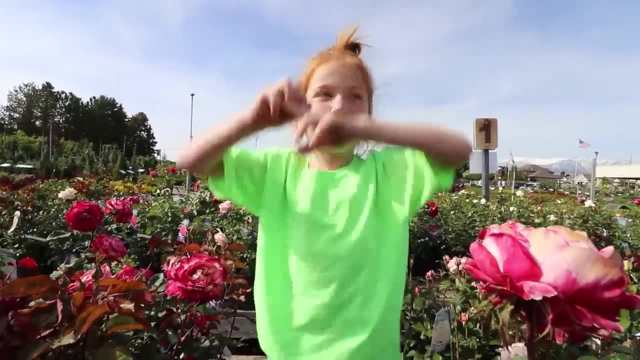 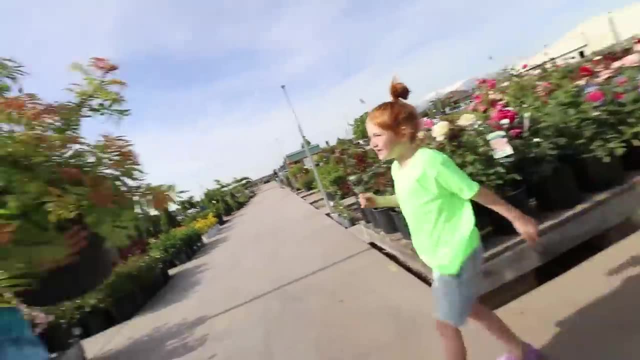 Today we're going to go grab some seeds from in there. Then we'll go to Parrot Island and plant them. It's going to be so much fun. Come on, let's go get Mom and Dad. What do you think about this one? 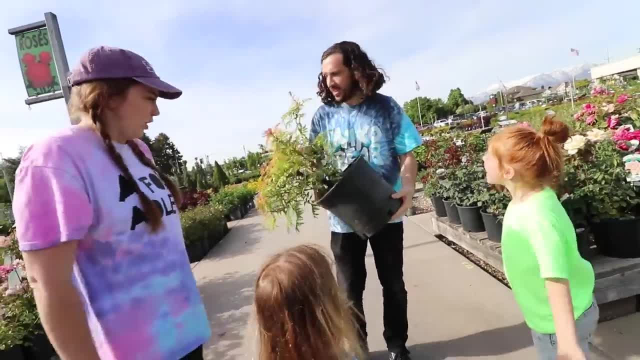 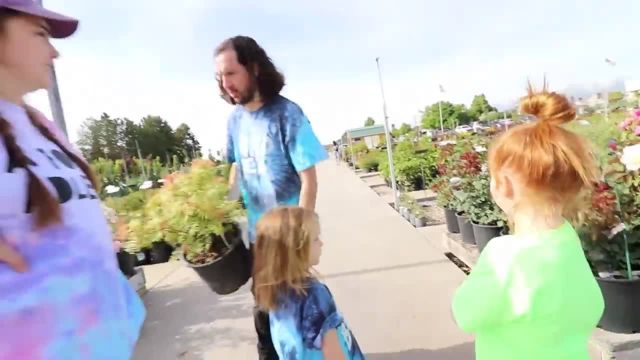 I wanted to plant our own seeds. You want to plant them. We're in the flower section, So you want to do seeds and plant them. I think they're in there. Alright, to the seeds. Dad put that back, Not getting that one. 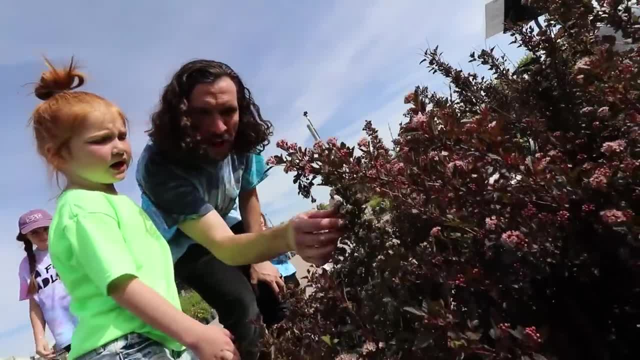 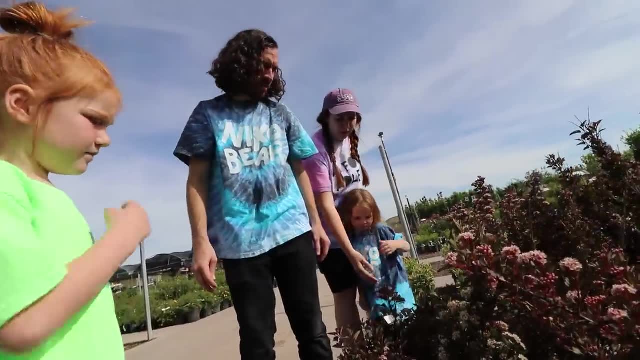 Dad, look at these plants. What are these? I don't know, but they have lots of little flowers. That'd be cool. I think I know these. We have a big bush in our front yard, remember, Mom? We do have this in our front yard, actually. 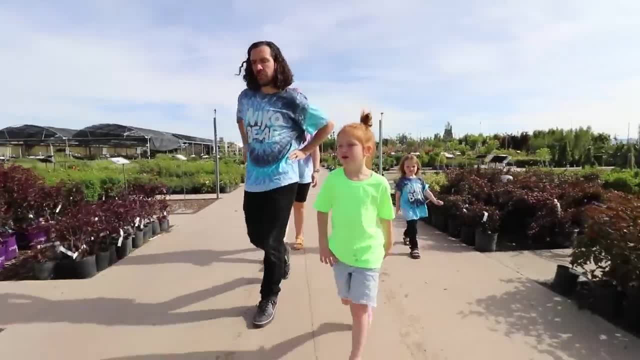 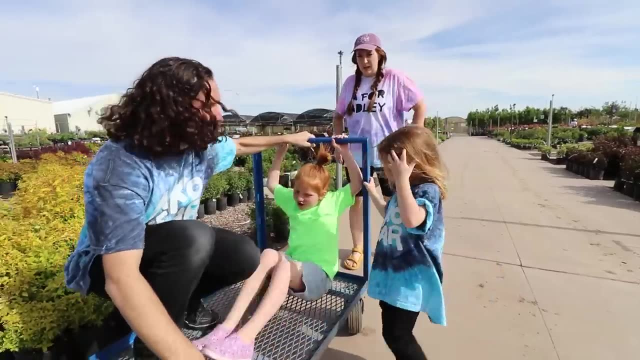 Like a big bush. Maybe that's why we like it. Where are these seeds you're talking about? We need a cart. I call being on the rider cart. I call being on the rider cart. I'm on the cart. Dad, you have to get off and push. 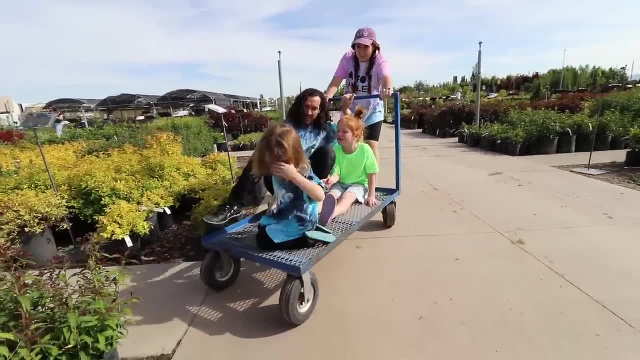 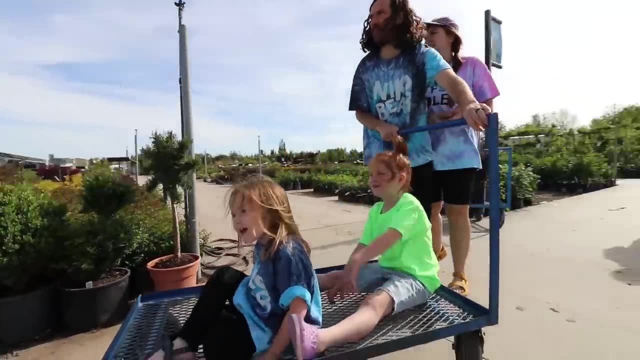 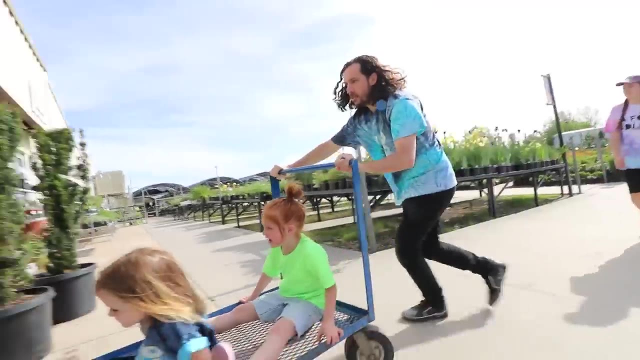 I guess I'm the pusher, Mom's the pusher. Oh wait, Dad's too heavy. We're only turning this way. Okay, Whoa, Alright, Stop seeds Trees, watch out, Alright, should we go inside? 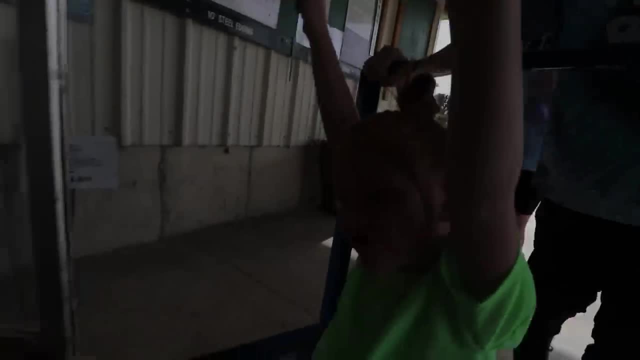 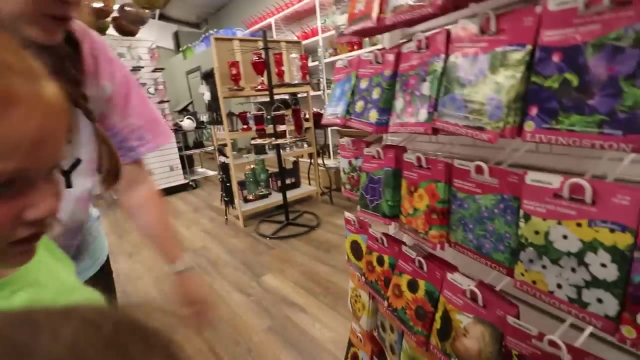 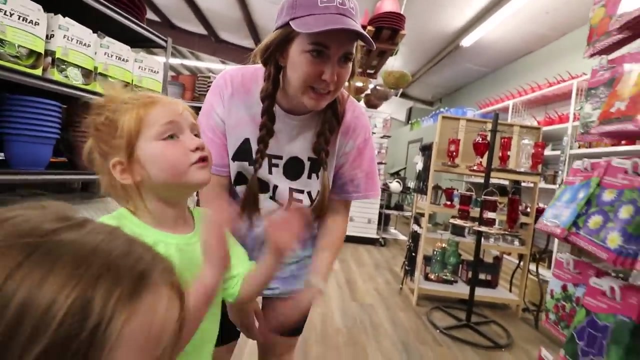 Yeah, Inside we go. Oh, I see the seeds, Dad, This is the perfect spot. Sunflowers, Those are pretty. Do we want to do flowers or do we want to do like watermelon carrots? Let's do both. 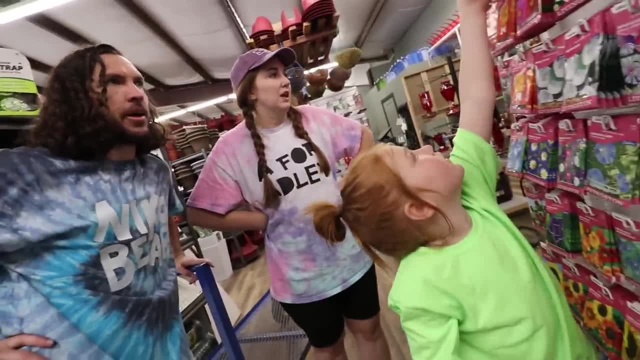 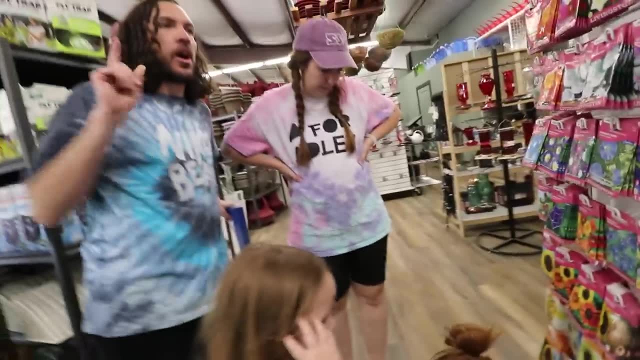 We could do a garden. How many places do we have to plant flowers? at Pirate Island I got four root beer barrels. We're planting our flowers in root beer barrels, So we could do a garden barrel with like fruits and vegetables and then a flower barrel with flowers. 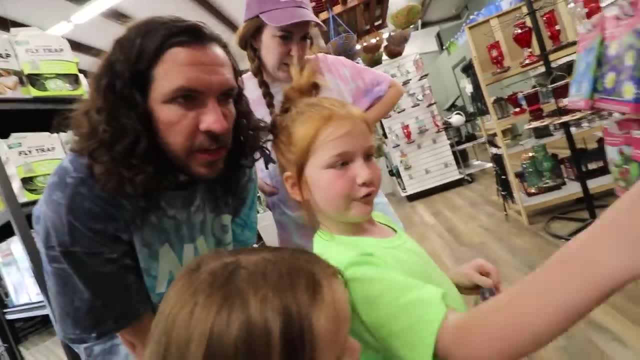 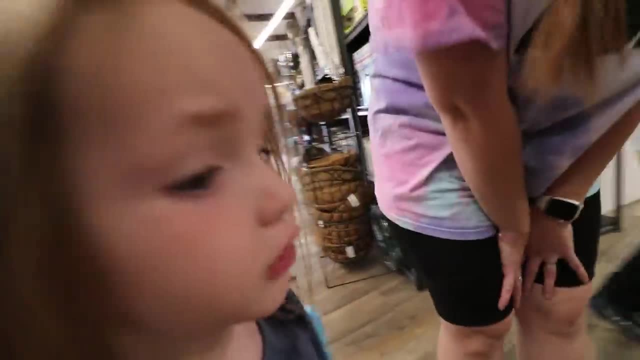 Okay, I'm picking some for the flower barrels right now. Okay, you go. What kind of stuff do you want in your barrel? Not these, Not sunflowers? Yeah, because bees don't enjoy flowers. and then we don't want bees that dink us. 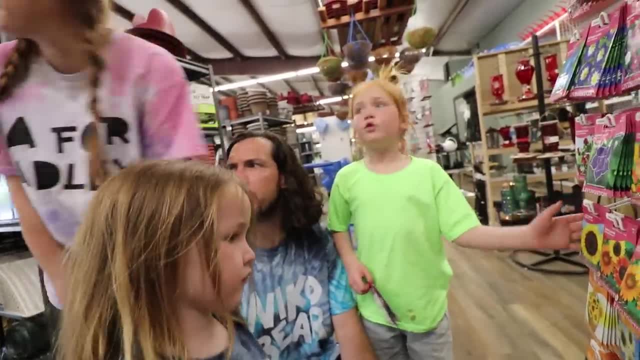 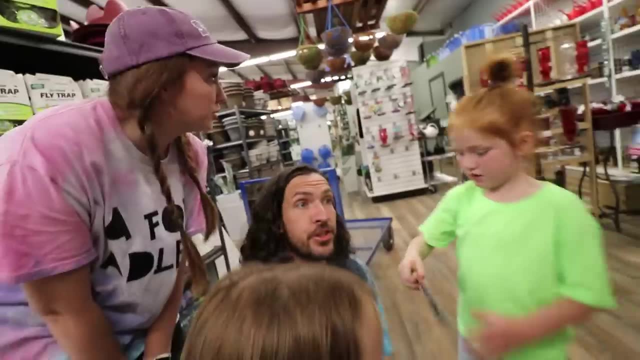 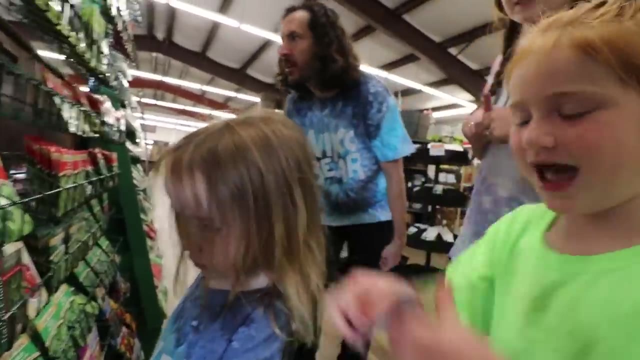 That's true. Where's all? like the fruits and vegetables, We don't want sunflowers, because the sunflowers grow really big and they would be super high. That's true. More seeds over there. Watermelon- Two packs of watermelon. I love it. 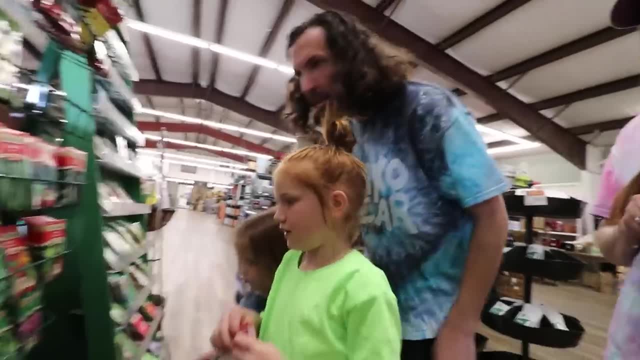 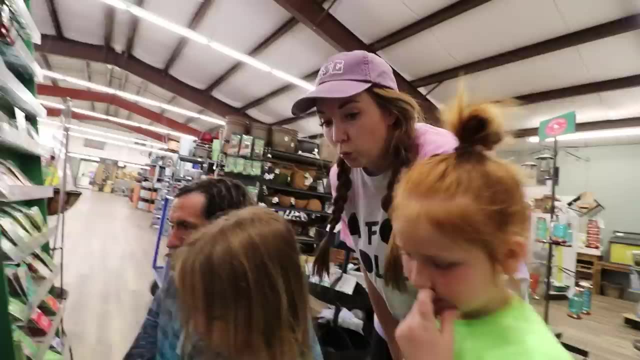 Corn on the cob Corn. I like corn. What else? Ooh, do we have carrots, Dad? these are pepper seeds, Pepper Hot. What if we get pumpkins? and then, when it's Halloween, we can carve them? That's actually a cool idea. 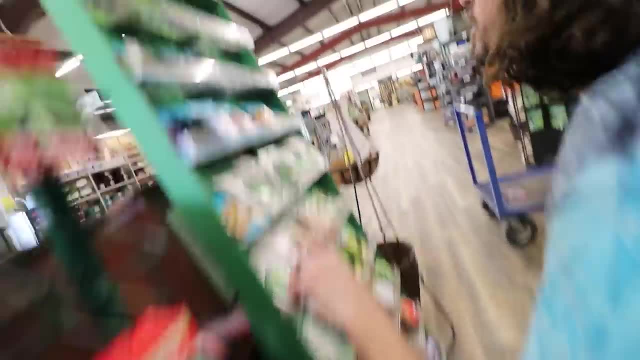 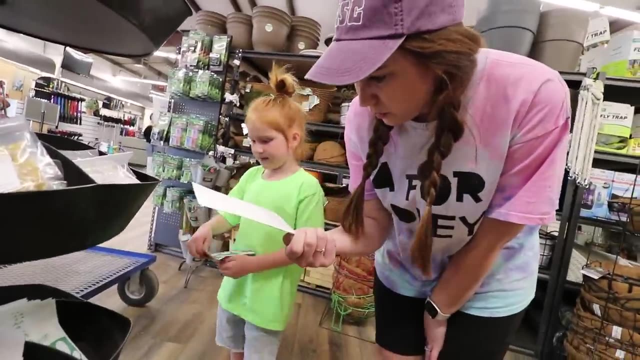 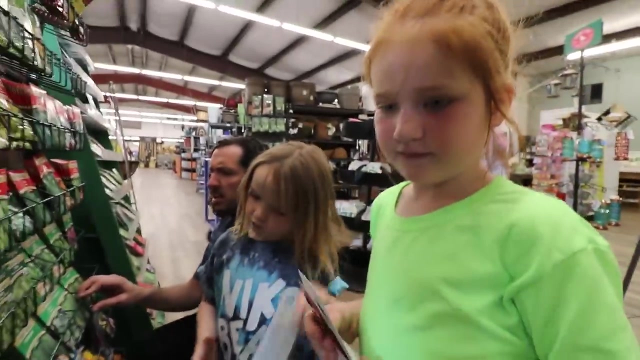 Do you guys see pumpkins, Pumpkin, pumpkin, Pumpkins. Oh, look at this, A Big Mac's pumpkin, Big Mac's pumpkin. Hmm, Ooh, celery, Ooh, that could be good. I want carrots. Where do you find carrot seeds? 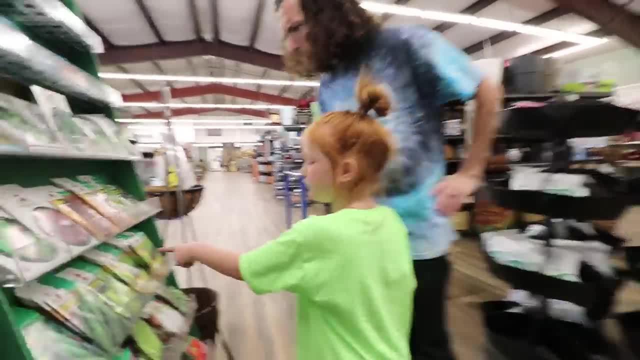 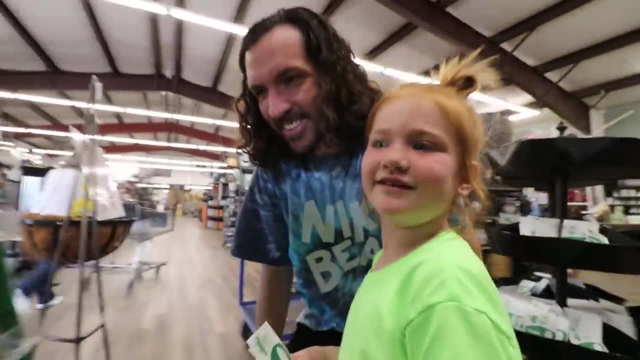 Or peas, That would be good Beans. I think those are peas. That's a cucumber. We could do cucumbers so we can like put them on our eyes and do spa days. Cucumbers- Ooh, what's this? Brussels sprouts. I don't think I like Brussels sprouts. Remember that's from Shark Dog. Oh yeah, Does Shark Dog like Brussels sprouts? Yeah, he loves them, But they make him fart. Is this a metal detector? 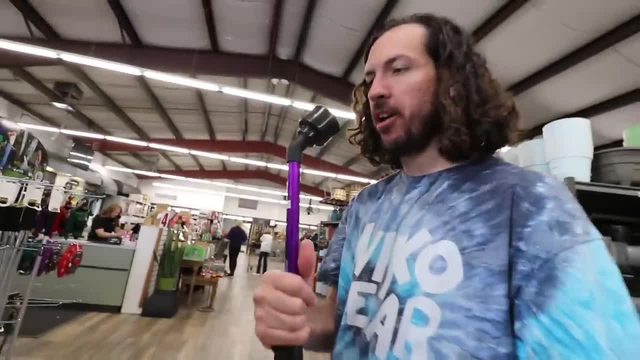 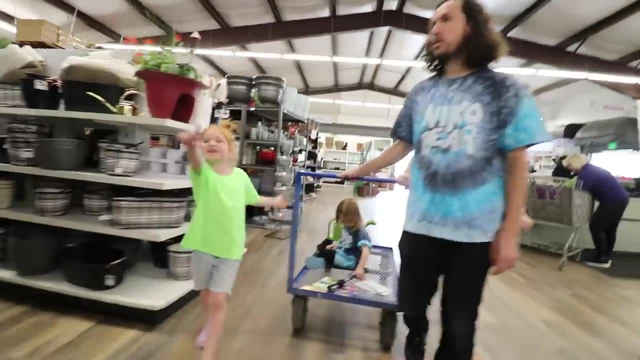 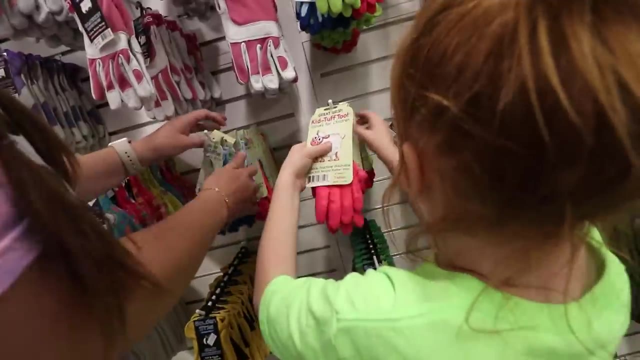 What the? I think I know what they are. You connect this to a hose and then Gardening supplies Over there. Gardening supplies, Ooh, gardening gloves. Should we get pink or blue or green? I want pink, Pink, okay. 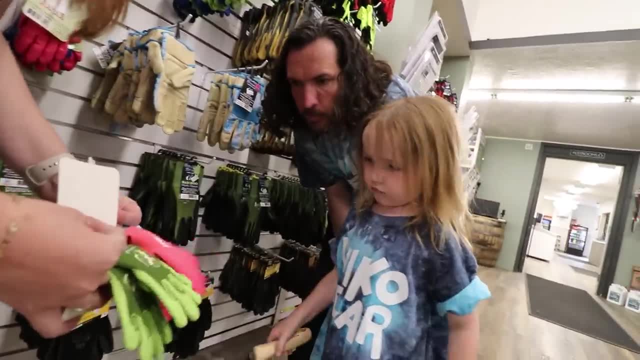 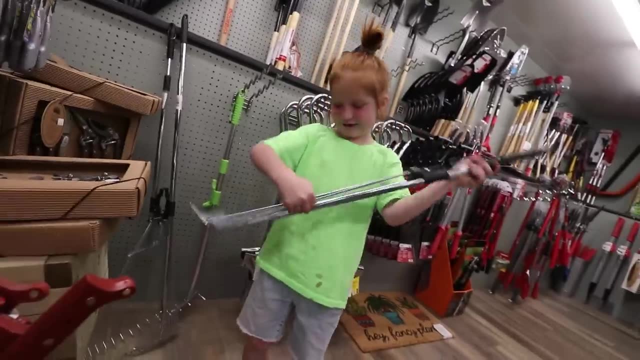 Which ones? Ooh, what ones you gonna get? Zebra, Yeah, Okay, Cool gloves bud. It's a money raker. You could play the guitar with it. Do-do-do-do-do, Do-do-do-do-do. 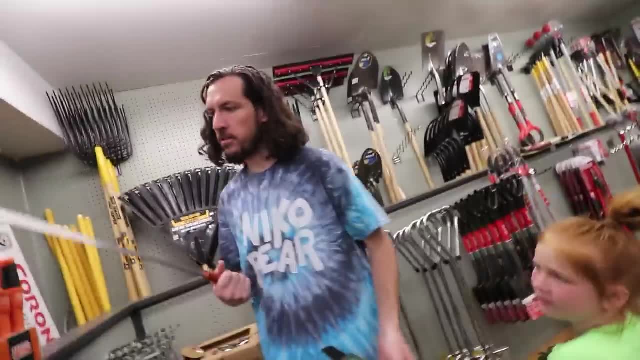 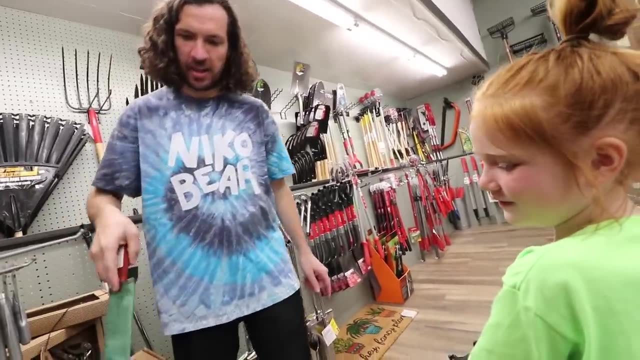 Do-do-do-do-do. Ooh, a machete That looks dangerous. I'm putting it away. What is that? It's a machete for like cutting down, like vines and trees and things that need to get cut down. Let's get it. 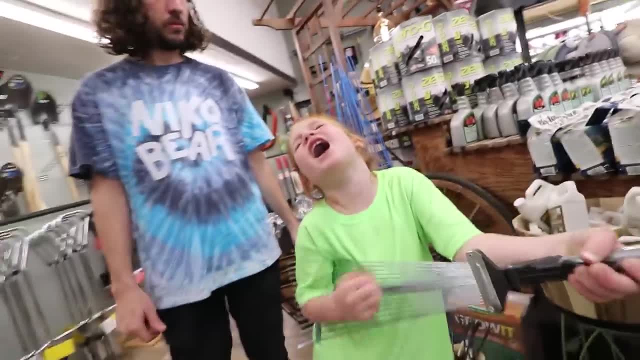 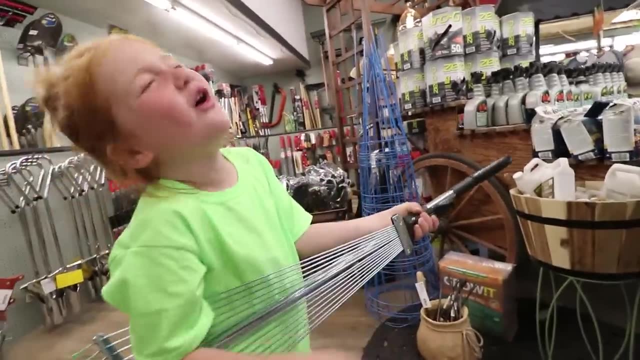 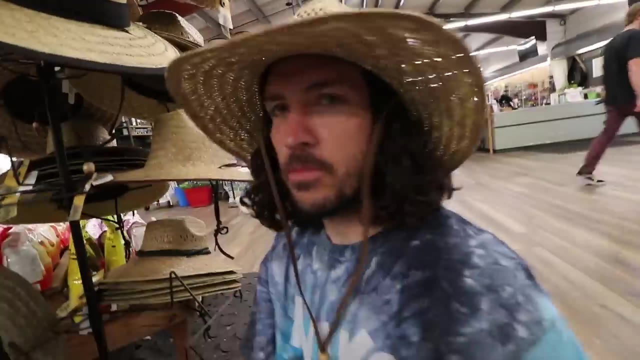 No way, I'm gonna show mom my new guitar. Mom, we got a new guitar. Whoa, Pretty cool. Welcome to A4A3.. Yeah, We got some garden hats. Do I look like a gardener or a scarecrow? Yeah? 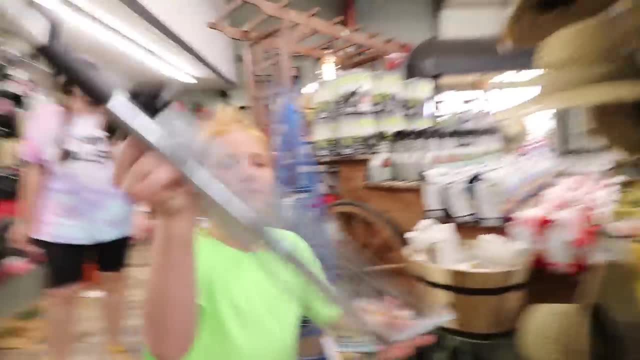 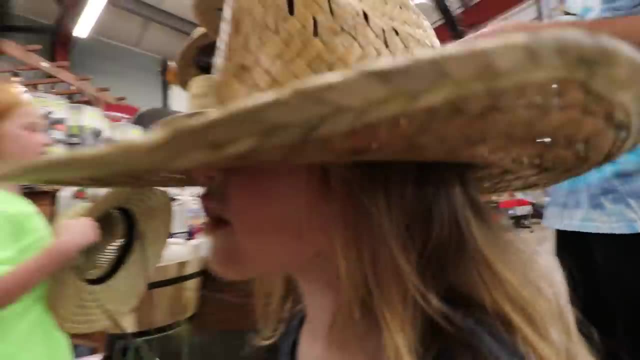 Do I look like a scarecrow? Yes, you do. Perfect, Dad play the guitar. Welcome to A4A3.. We're gonna plant some flowers So gladly. You look so good. I can't Adley. you wanna try one on. 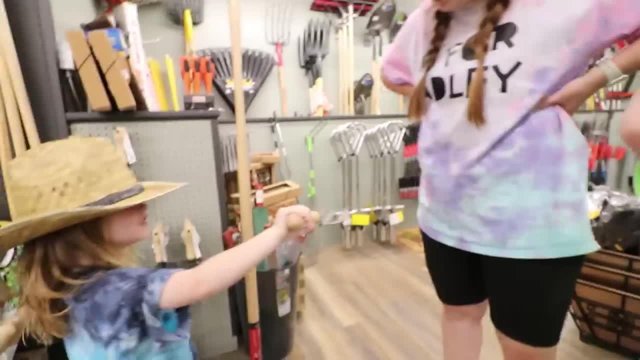 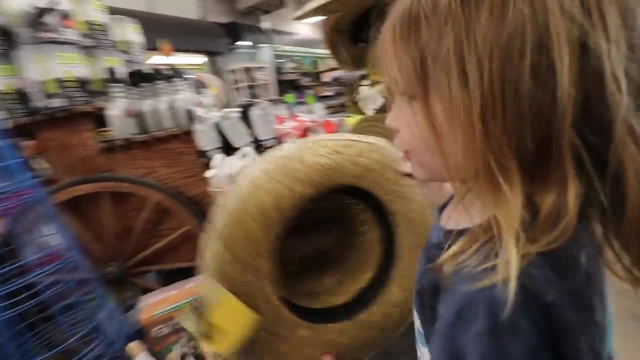 Oh, yeah, I like it. Oh, you look like a farmer. Alright, Guys, there's a whole bunch of flowers and stuff out there. Should we go check it out? Yeah, that's my good power, Yee-haw. 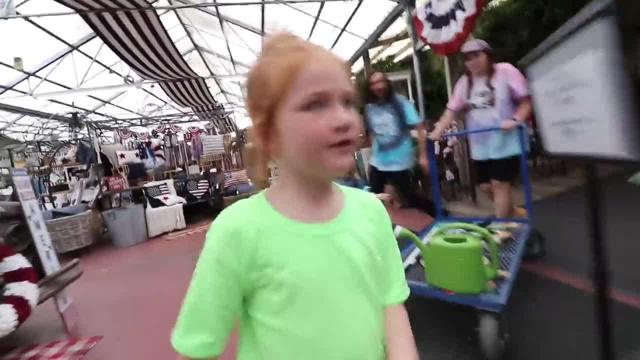 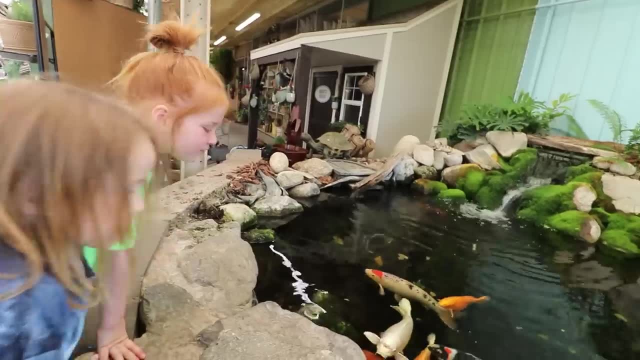 Come on, Niko, Let's go feed the fish. Wait, where's there fish? I'll show you Whoa they're big. They got big. Whoa They're like, right next to us, Like, can you guys bring food? 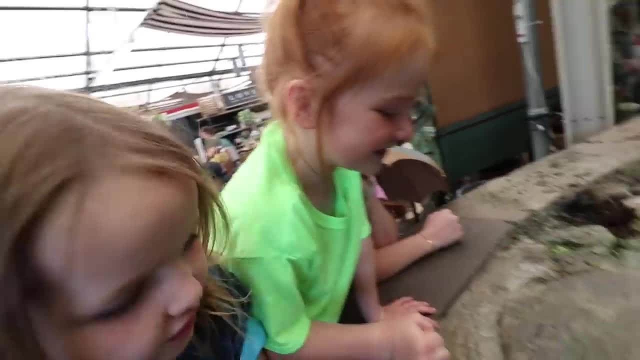 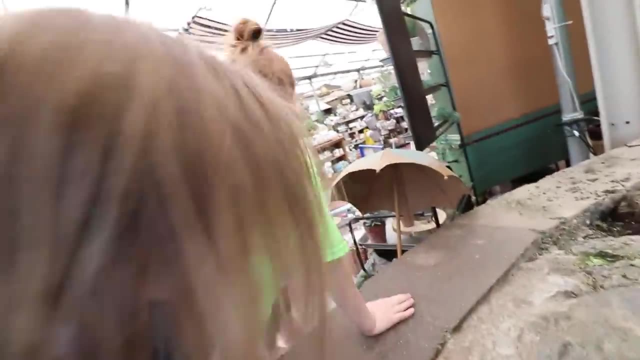 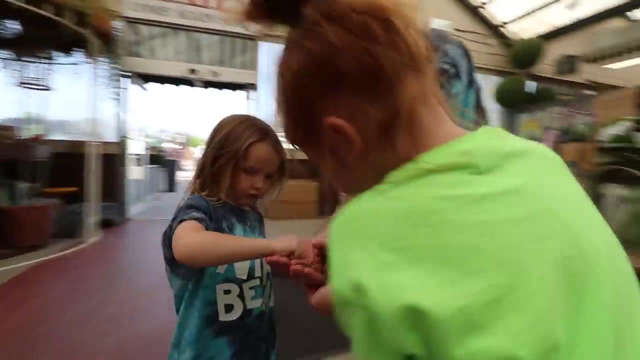 Okay, I'm just gonna quickly dip my finger in. Are you serious? Yes, Do it. I didn't touch it. I'm gonna get some food. I'll come with Bring food. I want some. I want some, Some fishy food. 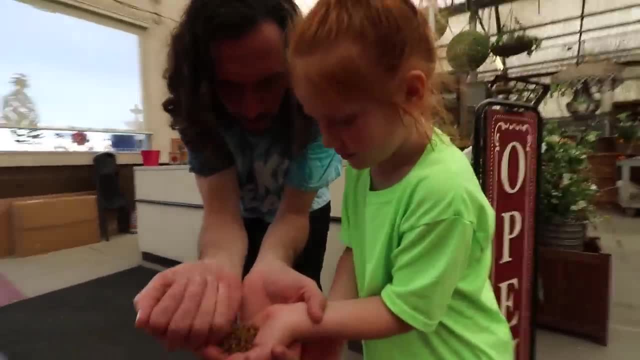 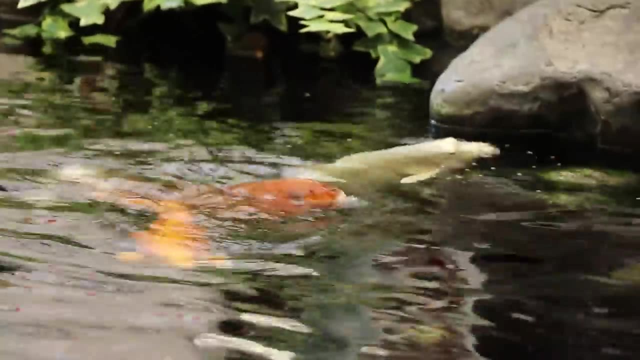 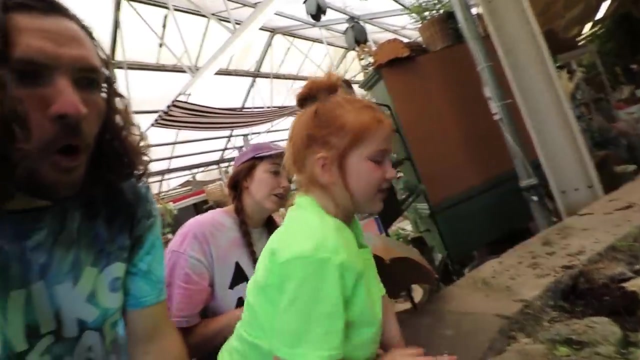 Wait, Oh yeah, They are gonna love that Here. fishies, Fishies, They love it. Ready for the jack frog vlog Here? wait, Oh, they are loving it. Look at that orange fish, He's loving it. 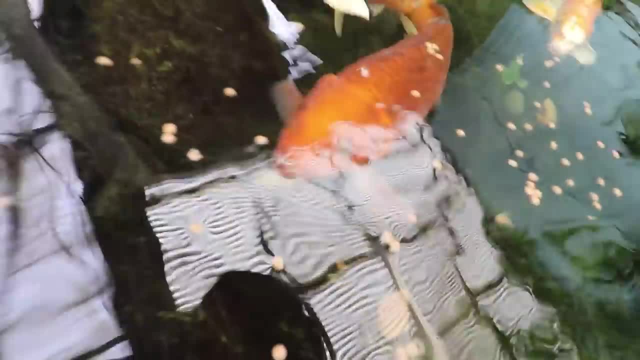 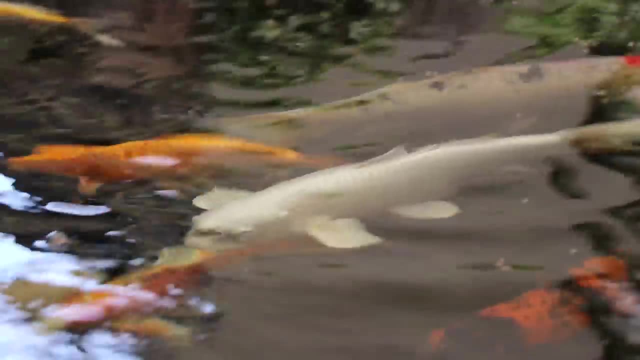 He's living the love time. He's like whoa, that looks Hope you like that fishies. All right, let's get back to gardening. Back to the garden, Let's go. All right. what else do we need? 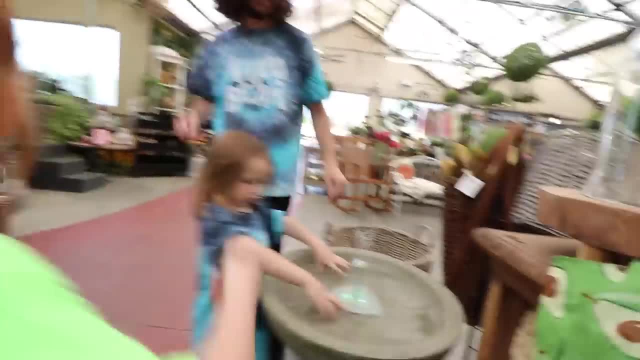 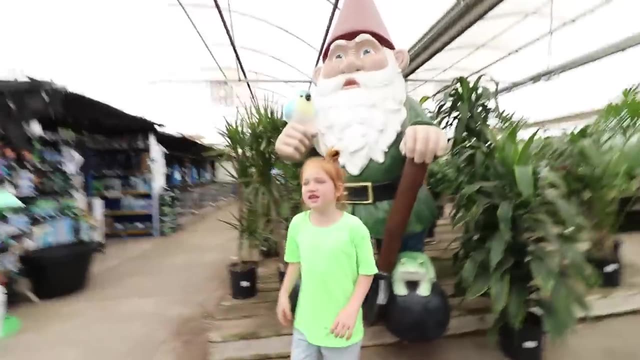 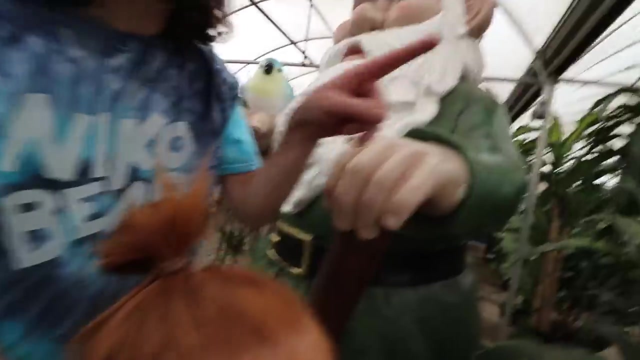 Just gonna wash my hands from the bird, Got some fish food Picture with the nose. Whoa, That is awesome. Look at this, Hello little birdie. Hello little birdie. Oh Adley, look at all this stuff. 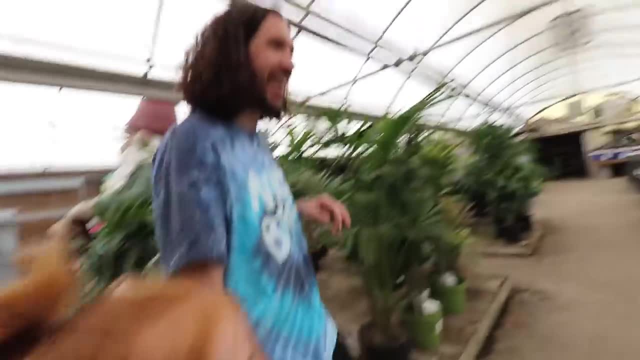 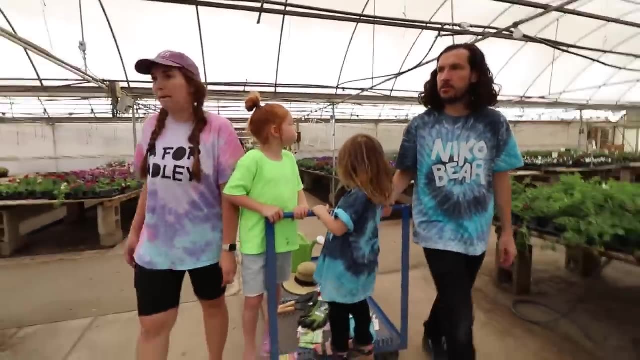 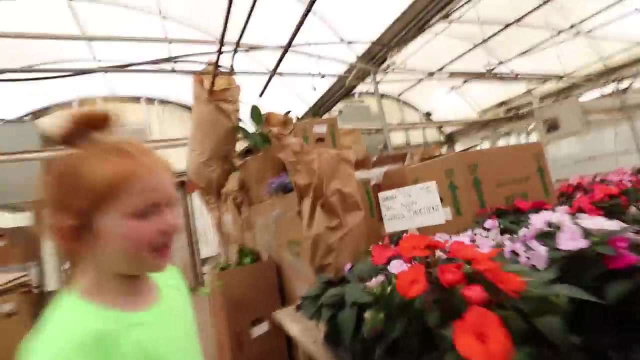 we can plant. That looks at me like a pirate. Do you guys want to get any of these flowers? Oh yeah, Do we want to get some flowers? Oh, I like this one. I like this one. How did you see that from so far away? 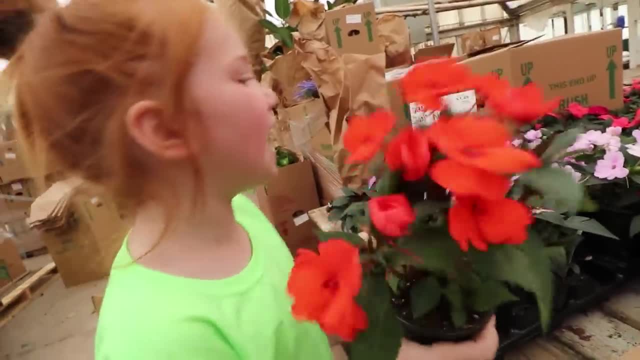 I know I love that one. Grab that one. This one- Yeah, I love that, And I also really like that one. Like this one- Yeah, that one, Let's go. We want these all. good, You like these Mom? 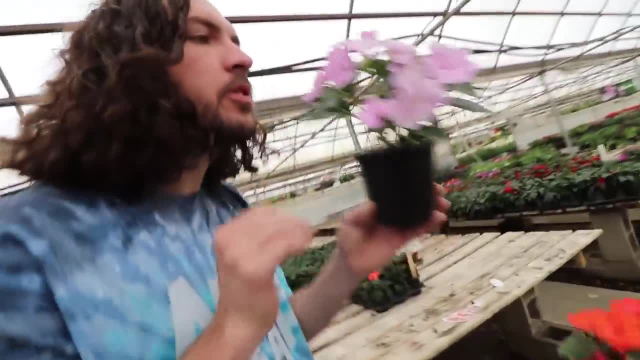 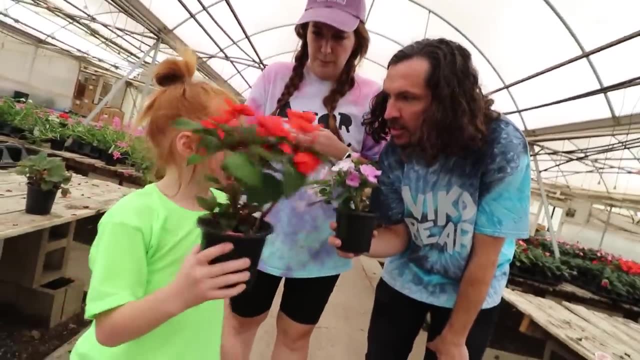 Yeah, These look like healthy flowers. I love little flowers, But I thought we were gonna plant them. We're gonna plant them, so you have to take them out of this and then replant them in the dirt at Pirate Island, Yep. So you can either plant a. 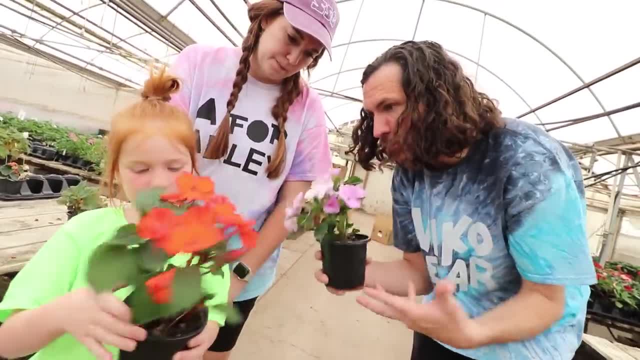 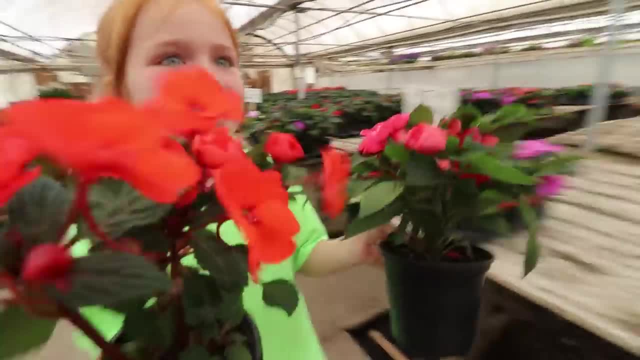 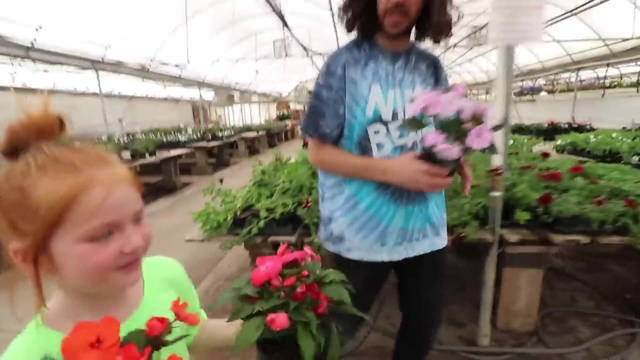 seed and have it grow, or you can plant a flower and then it grows more, or you can just plant a whole tree. Just grabbed another flower. that is adorable. Now you have one flower. Now you have two flowers. This one's cute. 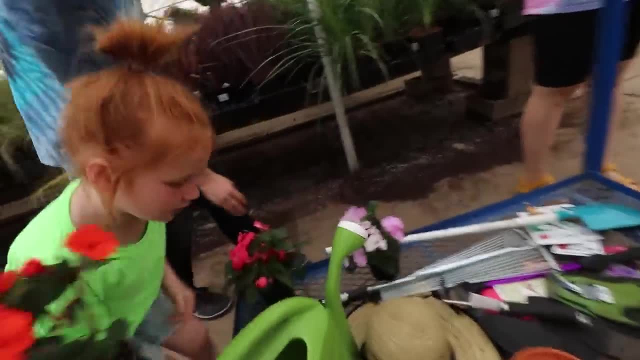 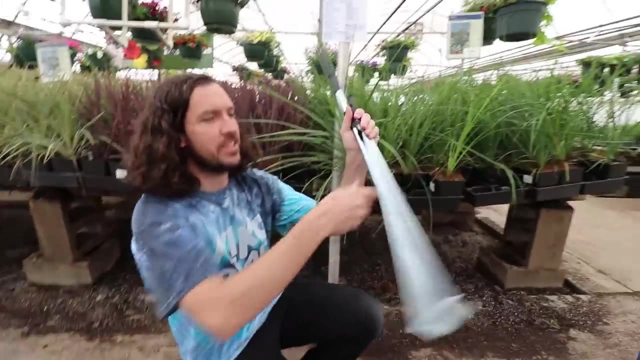 Mom watch out, Stop the cart. We got a flower delivery. We should clear things out. We need to go through our cart. Do we really need this guitar? No, We don't need a guitar. Goodbye guitar. Let me do one more guitar thing. 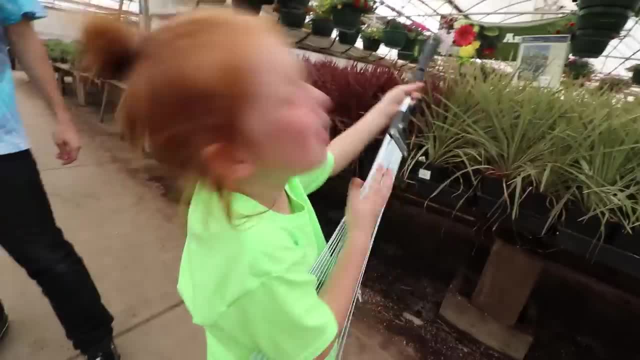 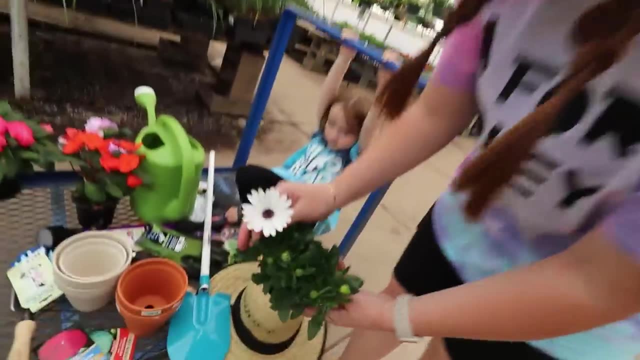 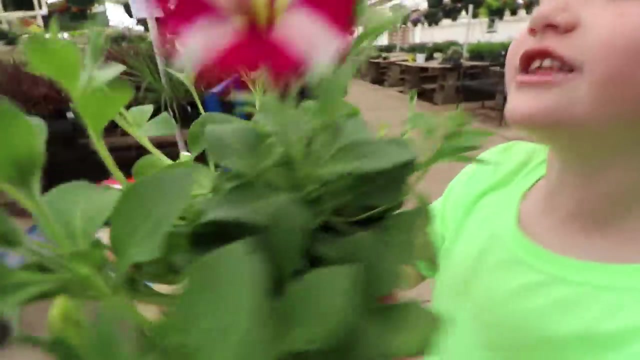 I love you. guitar. I will miss you. guitar. Mwah Bam, I found one I want to do. It's white and has a purple middle. This one's adorable. That one's pretty Dad. look what we got. 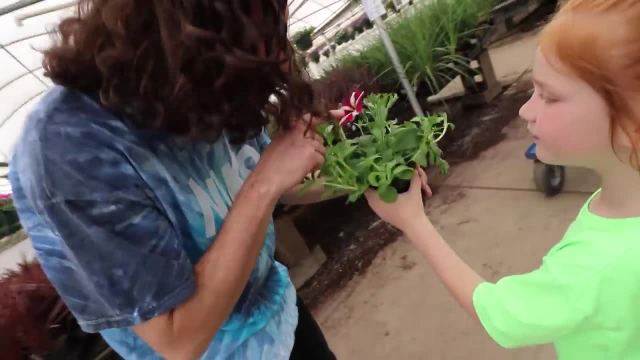 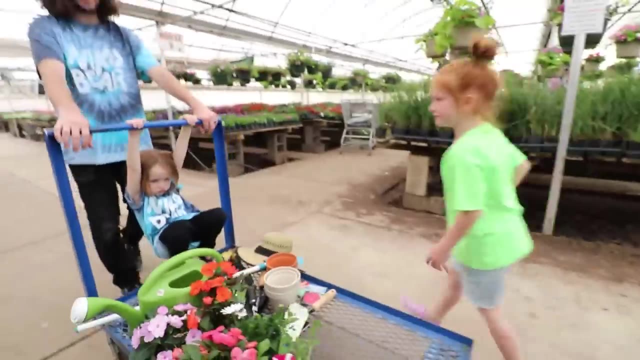 Look how cute That's like a little stripe flower, A zebra flower, And we also got this flower. Ooh, is that like a daisy? I don't really know my flowers, but I'm working on it. You lost a hat. 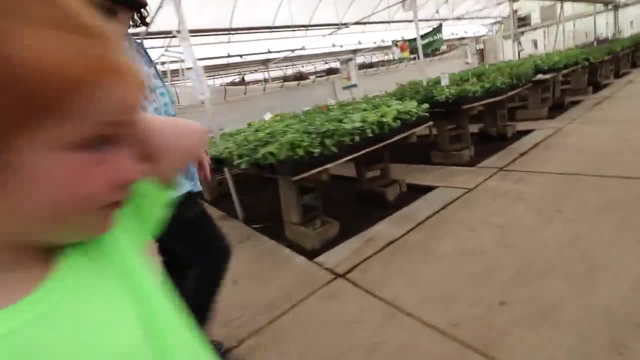 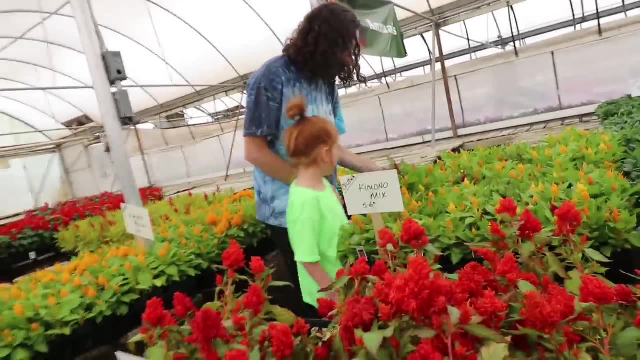 Mom's hat Hat overboard. Those ones are like paintbrush flowers. Come look at these. It's called a castle orange. I like the pink one. They're pink and orange mixed. Ooh, I like these. Should we do something like that My teacher gave us? 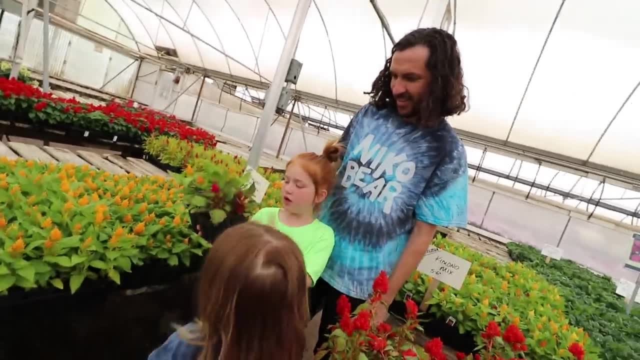 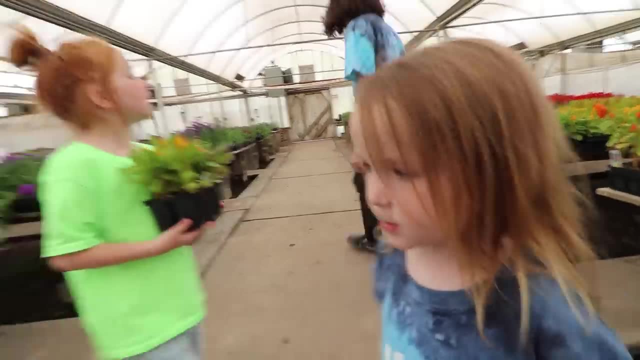 these. My teacher gave us these and then we put them in a and then she cut like this out, And then we brought them home. Really That's cool. And then I also got lettuce. I want to buy these. Are these snapdragons? 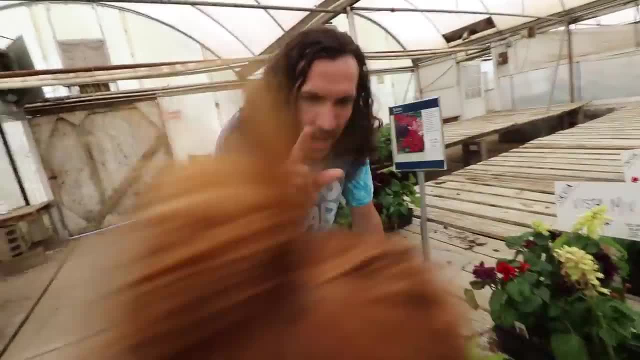 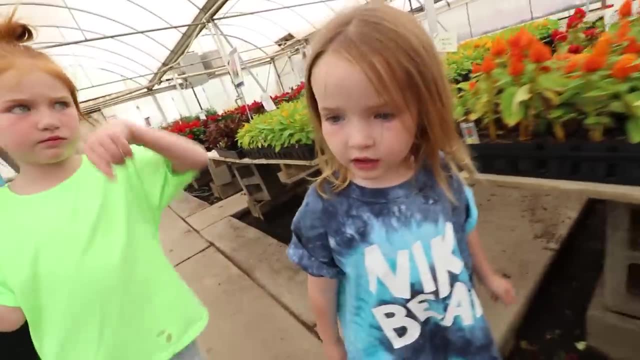 What were you looking for? There's like a flower called a snapdragon and you can put your finger in it and they look like little dragons. I used to like them when I was a kid. If you go inside the flower then you'll be trapped. 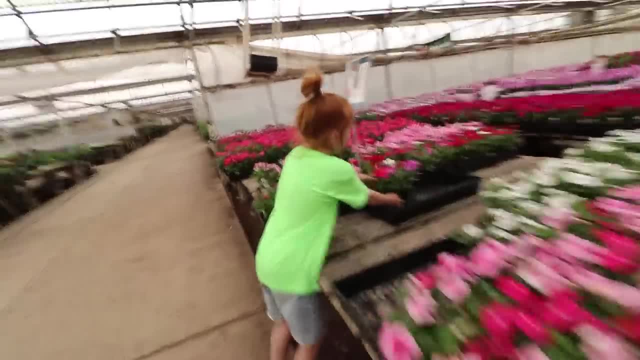 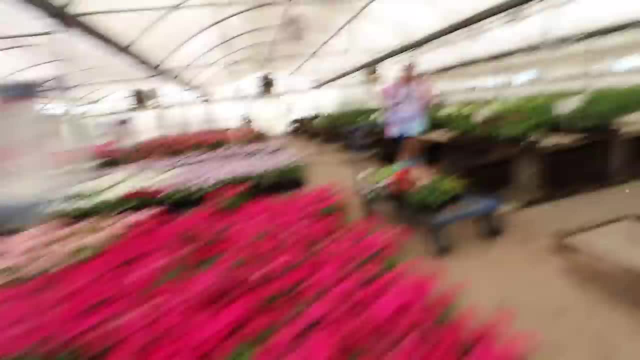 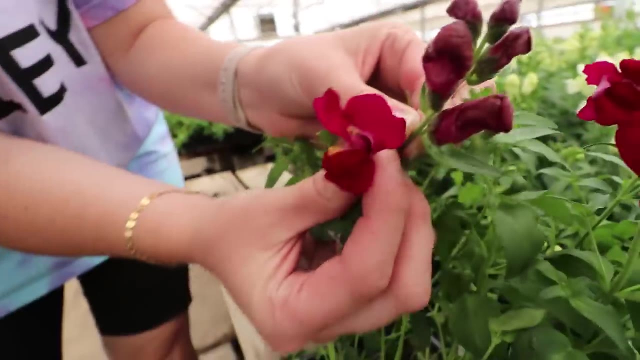 These are dragons. Oh, these are adorable, Daddy Aww, And they smell good. I found them. Look, Welcome to the best day ever, Hi Adley. Those are the snapdragons. Do they snap you? No, 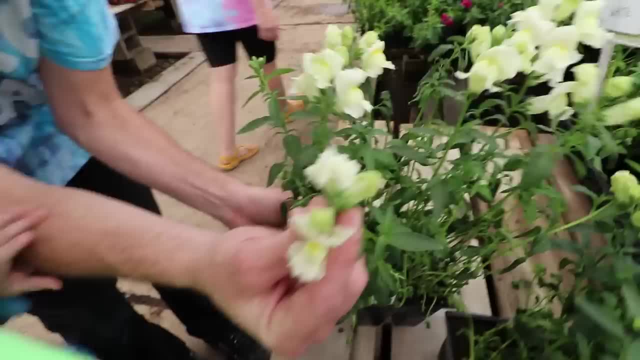 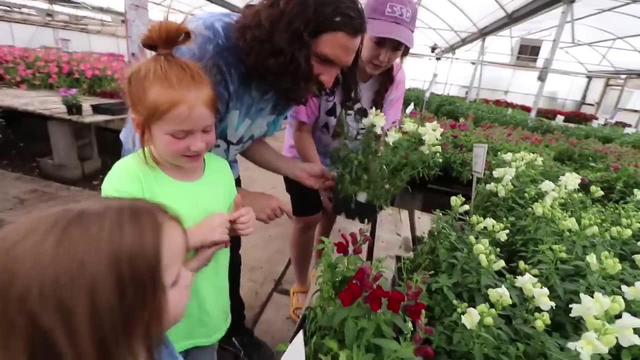 No, they're nice. Oh, and there's white ones. They have all different colors. Hi friend, It has teeth, Ooh, flower teeth. Should we get snapdragons? Which color should we get? Let's get the white red. 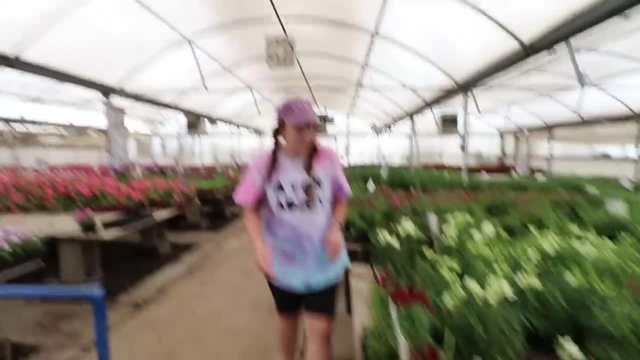 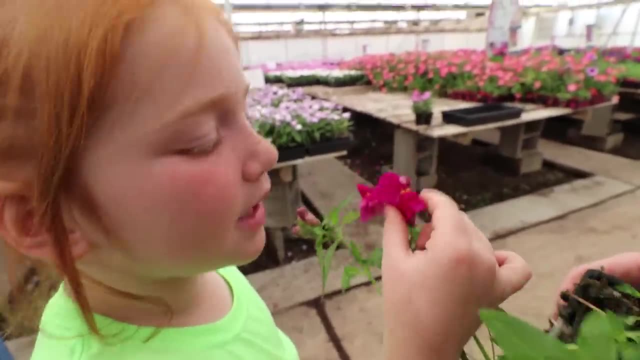 pink, purple- I want to get pink. These ones look pretty. What do you think about these ones? Oh yeah, these ones, Please buy me. Please buy me. Go plant me at Pirate Island. Alright, sounds like that flower. 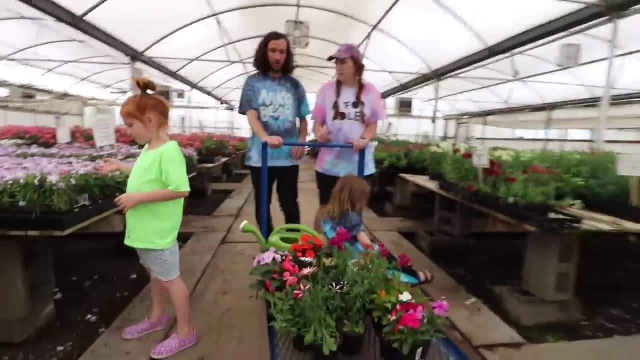 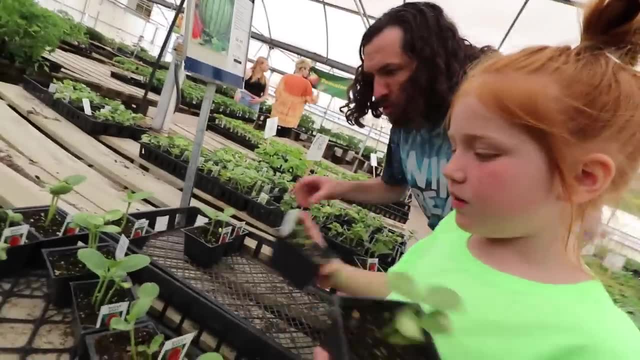 wants to be planted at Pirate Island? Alright, here we go. I think we have some good flowers. I'm still looking for my carrots. Watermelon- Oh, grab one of those watermelon guys. Me and Niko can plant our own. 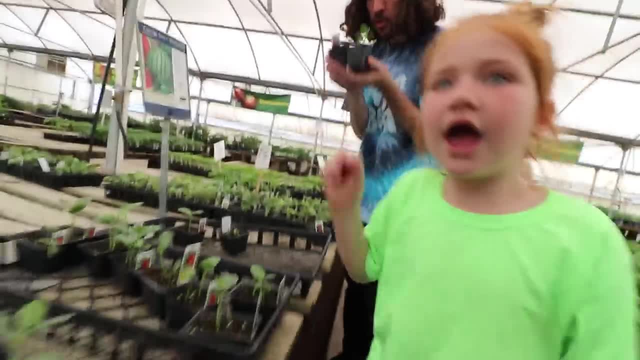 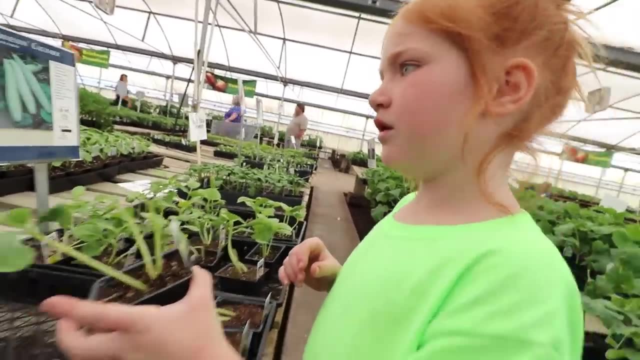 Dil, I like this one, This one and this one. Yeah, You guys are the winners. And then there's oranges over here. Wait, are these lemons? Lemon cucumber? I thought there, I thought there was more oranges Like lemon cu-. 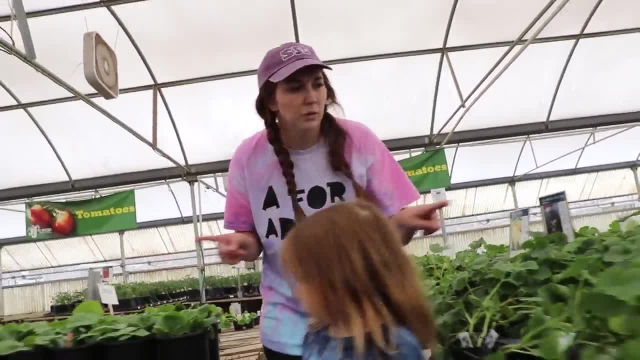 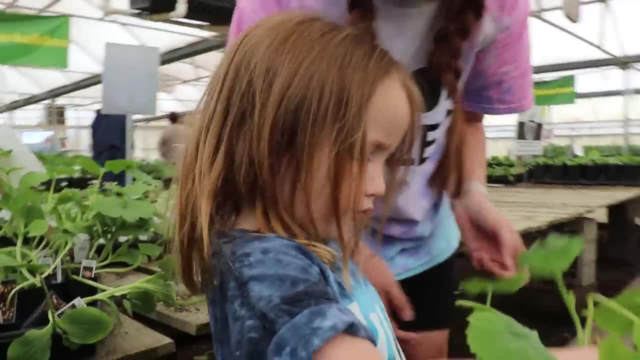 I know where the pumpkins are. You do Pumpkins, So do we want a medium or a large pumpkin? Medium, Medium, okay, This is mine. It has a seed in it. Look, there's a pumpkin seed. 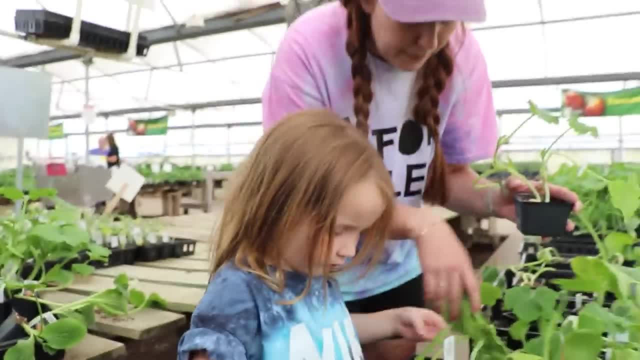 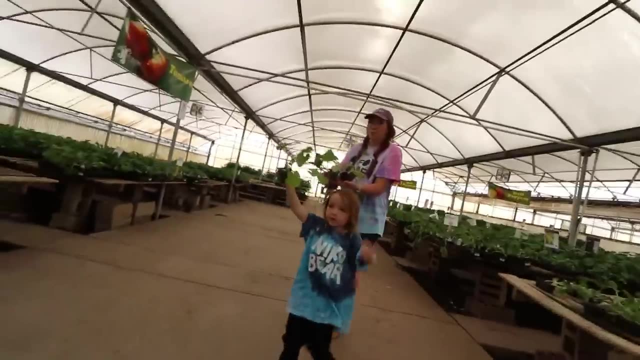 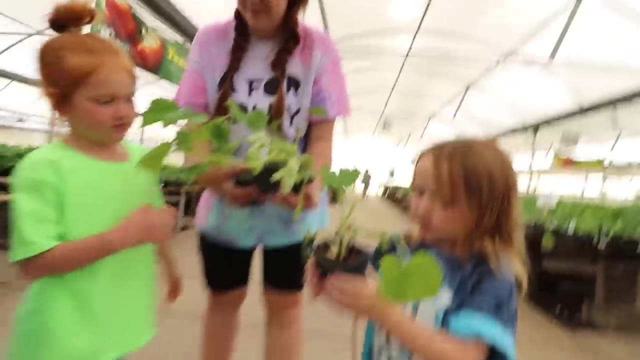 These are maybe an ugly. Okay, Ah, maybe dropped. Alright, I got this one, This one. We got some pumpkins. We got pumpkins. Those are pumpkins, Yep, And then we can carve them for Halloween. These are mine. Okay, those are your. 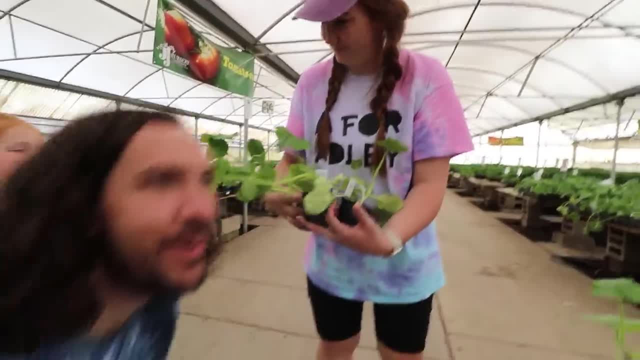 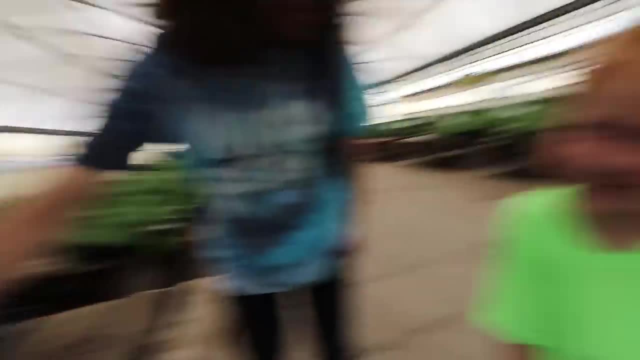 pumpkins. We got one for Niko, Adley, Navey and Mom and Dad. Perfect, Okay, one. Mine is crazy, I think those are oranges. Uh, those are not oranges, Those are tomatoes, Are you crazy? 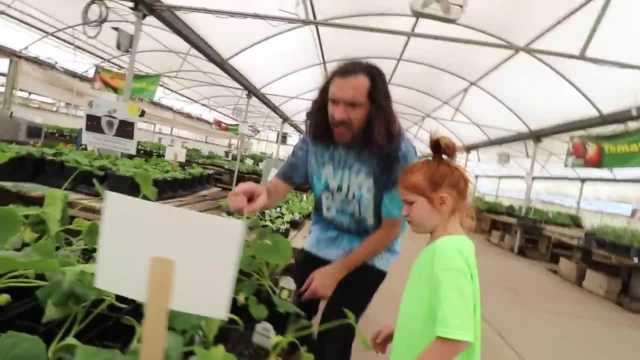 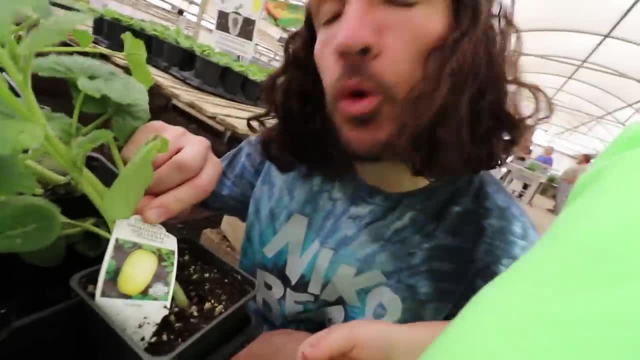 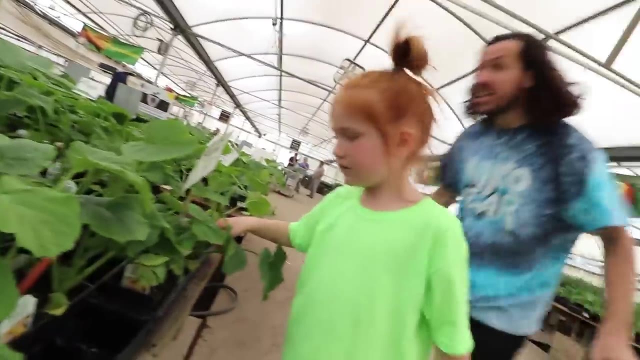 Wait, spaghetti Spaghetti. It says these plants grow spaghetti. Oh, spaghetti squash. Ah, Wait, what's this? Pink bananas, Pink bananas, Pink bananas. I want one, I want one, I want to grow pink bananas. 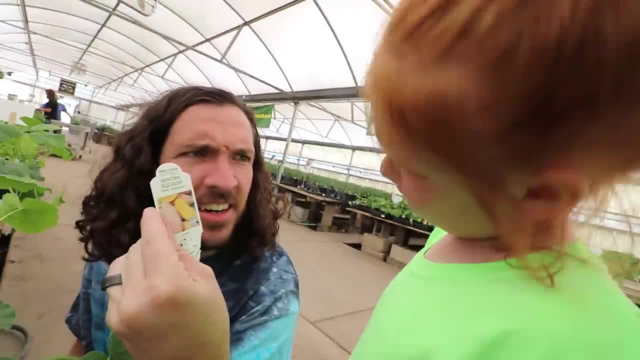 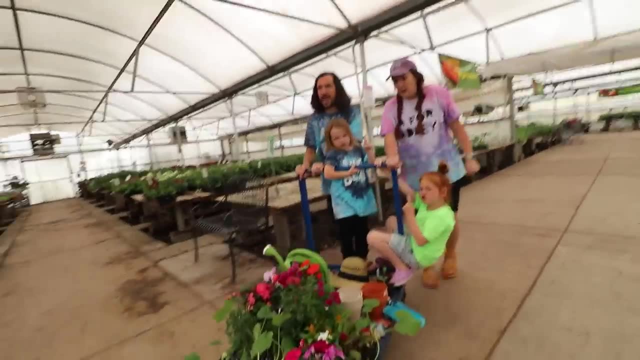 What are the pink bananas? I don't know. That does not look pink. Yeah, I don't believe it. Let's go to Pirate Island to plant our plants. Are we ready? We're ready, I think. Whoa, we're on our. 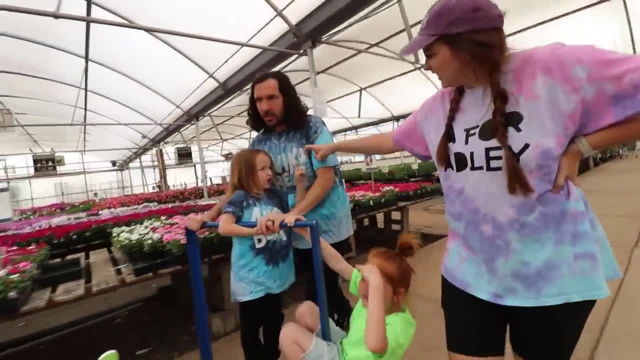 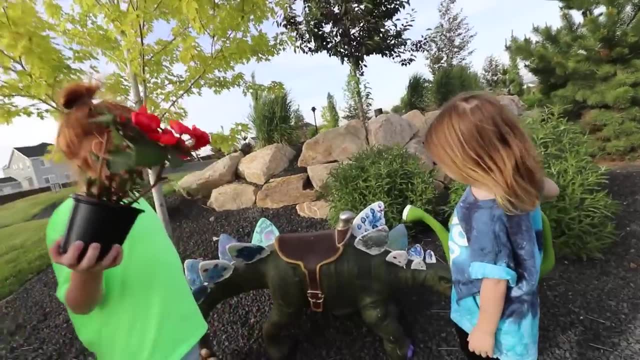 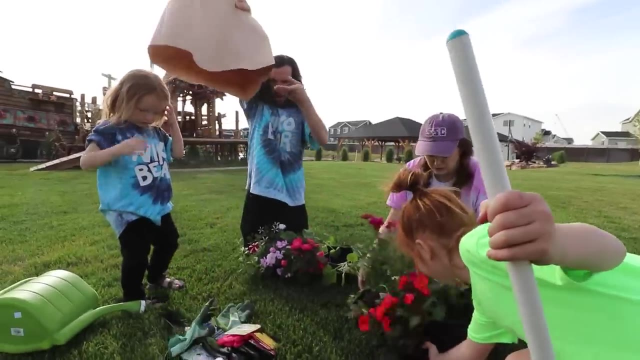 way to Pirate Island. Let's plant some flowery flowers, And then we have some other ones. Niko watered a dinosaur. Hi, dinosaur, Niko's watering it. Okay, All our stuff Are all these ones flowers, Look. 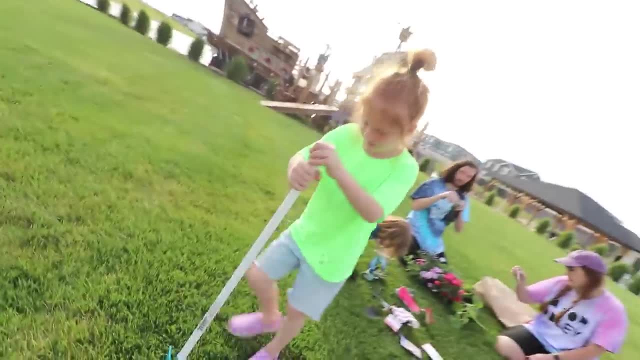 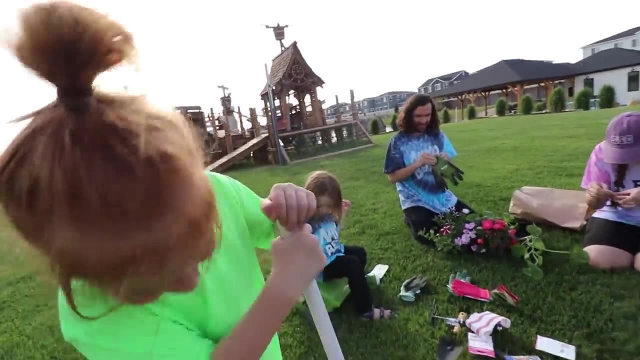 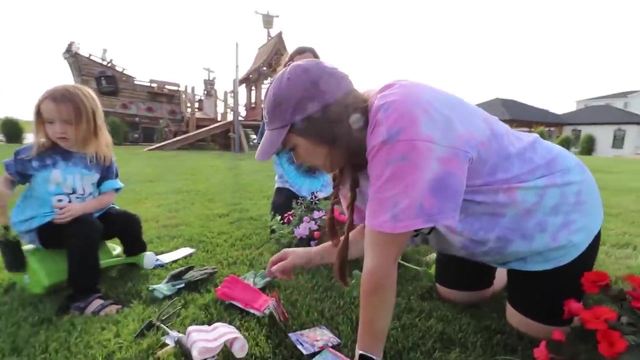 Look, I think we're going to plant right here. Wait, Hey, no, digging up our Pirate Island. I thought we were planting plants. Yeah, Okay, Where's everyone's gloves? Glove, check Gloves, Mommy's gloves, My gloves. 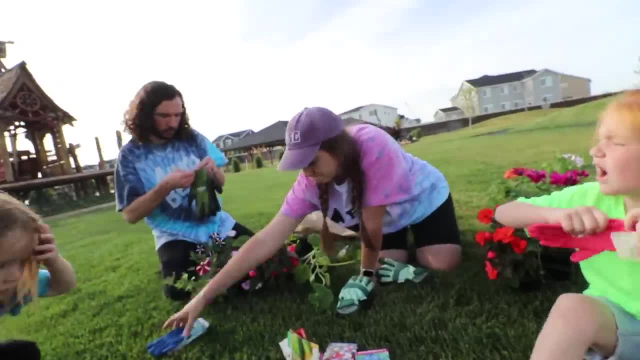 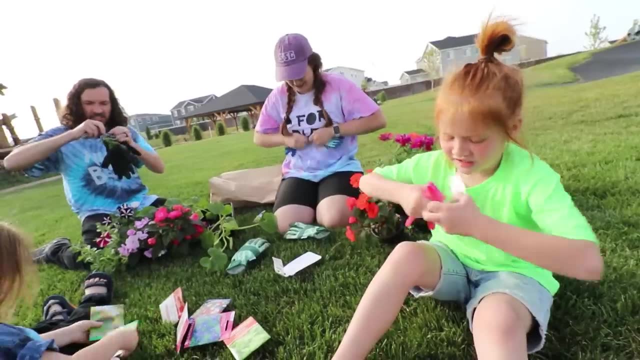 Niko, you got gloves. Do you want me to open them? No, I don't need help, I'm best at open. space station style. Hey, Space station style, Yeah Yeah, Garbage in the bag, Garbage in the bag. 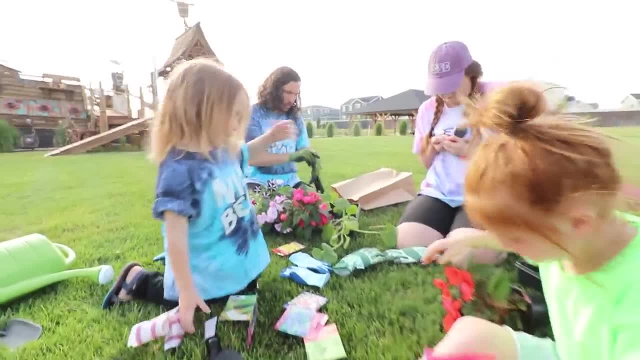 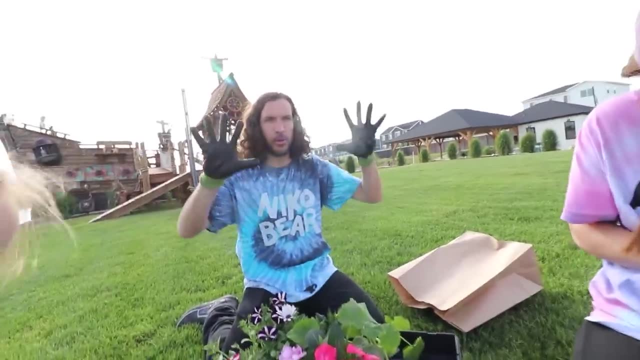 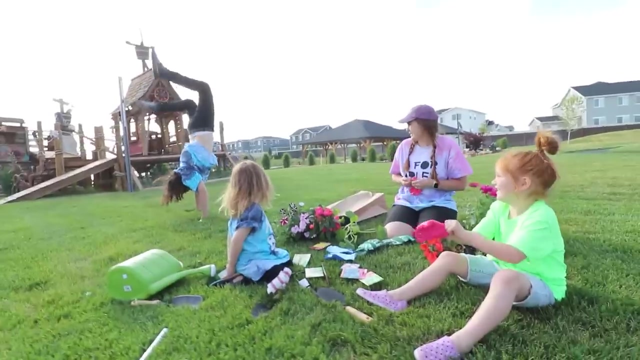 Okay, Niko, gloves. I got watermelon seeds and purple flowers. Okay, I've got my gloves. Do you know what these gloves are good for? Gardening? Nope, Handstands, Hands up, They work. It's hard to put my gloves on when you already. 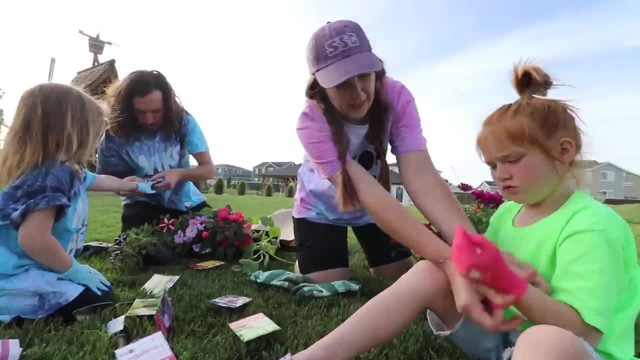 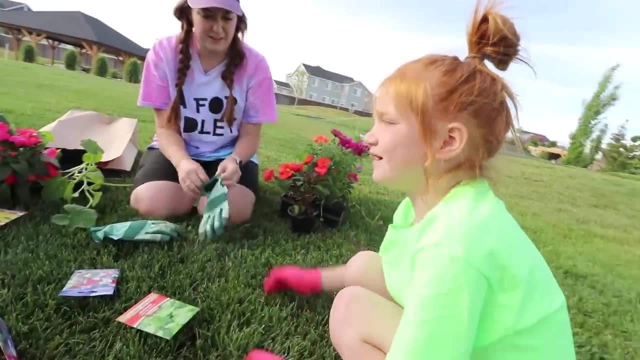 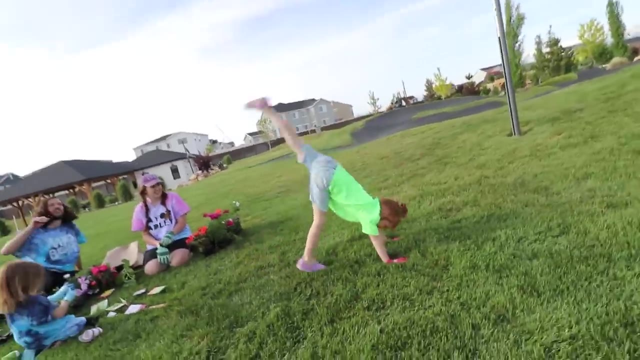 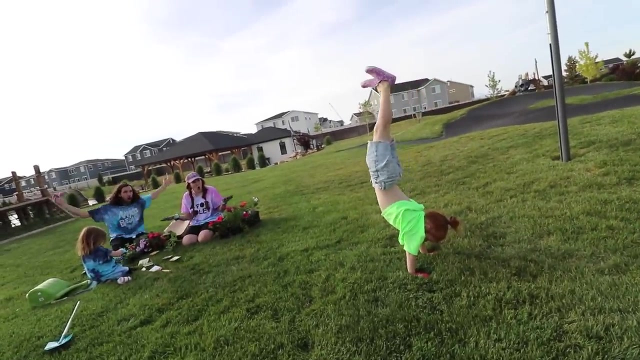 have a glove on, You look like you're a doctor. Dr Adley is ready for planting. Do you know what these gloves are good for? What? Yes, Gardening, Yes, but also handstands- Good job, What. 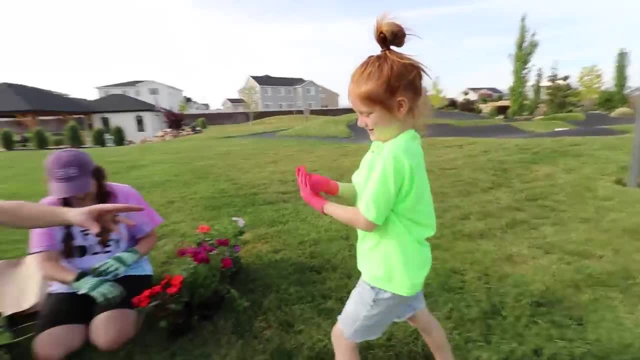 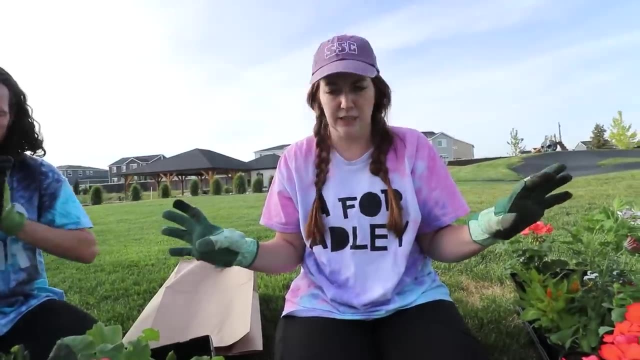 What? Let me see those gloves. No, Those are like extra grippy. So we have two planter boxes here that are in full sunlight, and we have vegetables here that need full sunlight- Full sunlight, Perfect. So we have watermelon and pumpkins that need full sun. 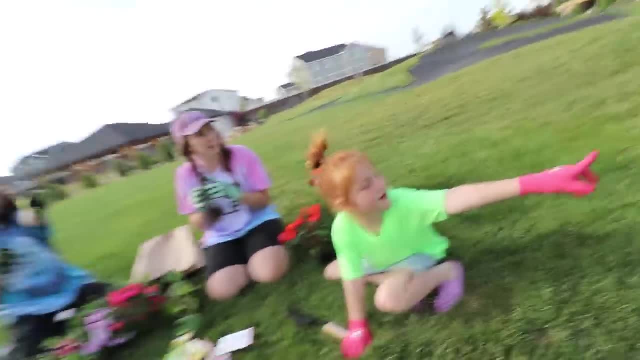 Where do we want to plant the watermelon? Oh, over there by the dinosaur. Yeah, watermelon by the dinosaur. Okay, me and Niko, Do you know where the watermelon is? Which one's the watermelon Watermelon? 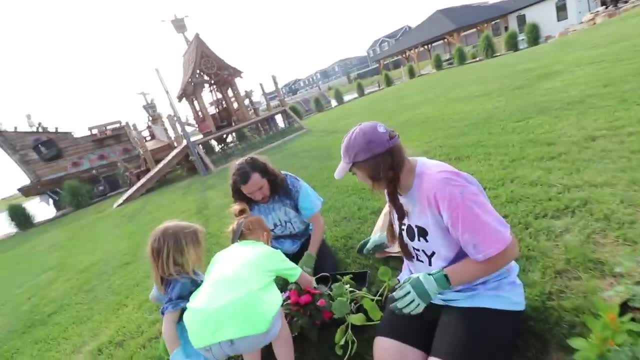 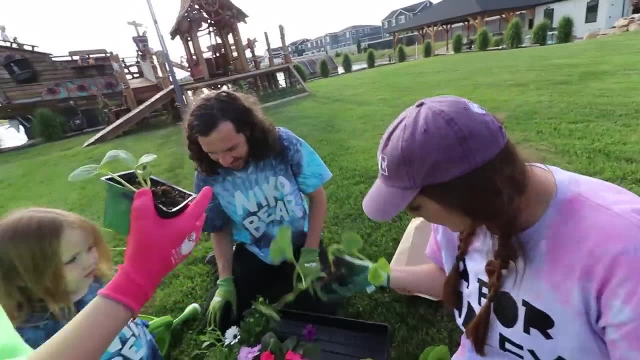 Those are pumpkins. Those are pumpkins. Where's the watermelon? Are these the watermelons? No, no, that's not Careful. they're friends, They're holding hands. You guys cannot grow together, Okay. 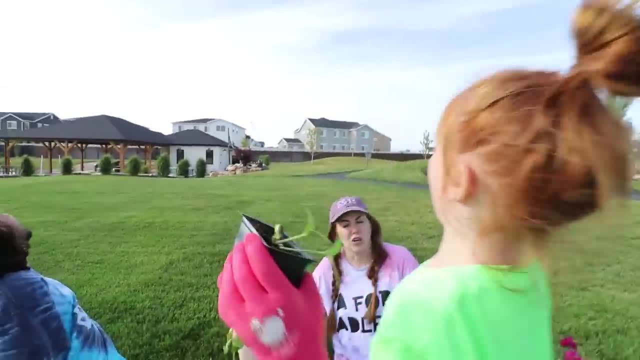 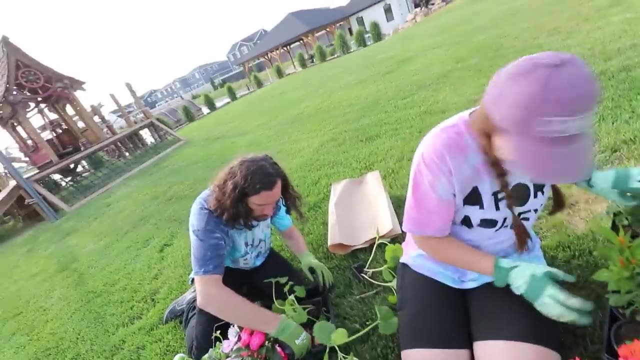 Ah, Niko just went like this and she said, yeah, Yeah, That was. How many watermelons did you get Two? Where's the other one? Oh, here it is. Maybe watermelon Niko, here's yours. 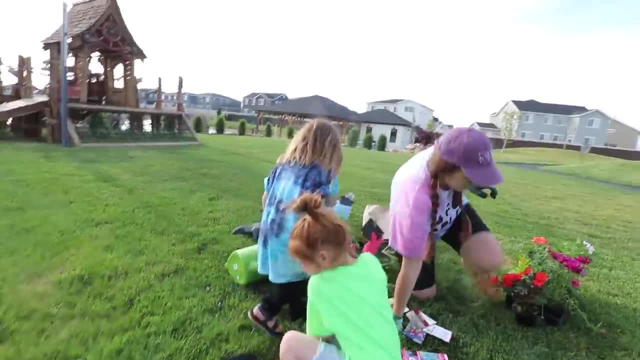 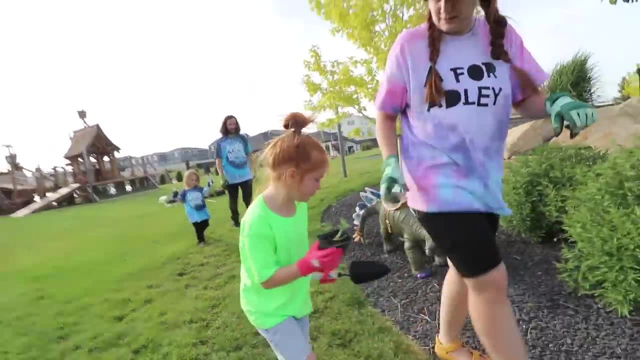 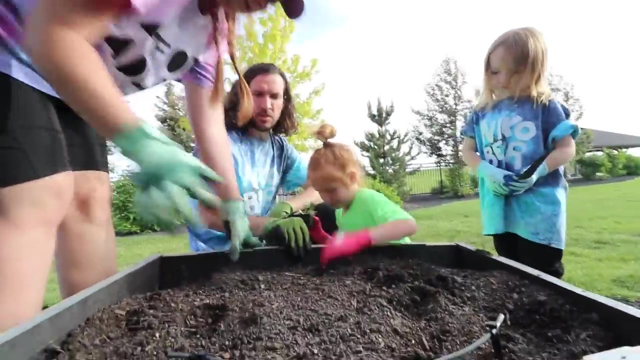 We need shovels, Shovels, Shovels. Let's go that way. Alrighty, Good job, I'm gonna dig up some treasure. Probably need to put one right here and then one right here. okay, I like those two. 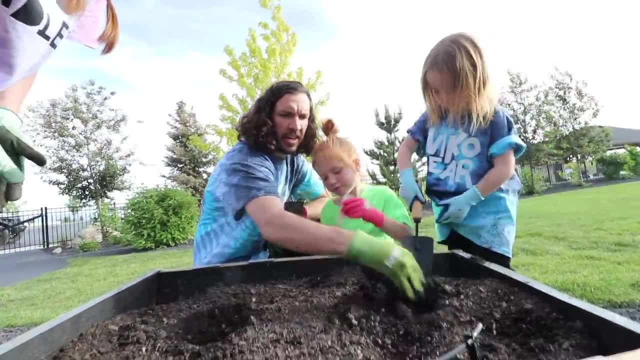 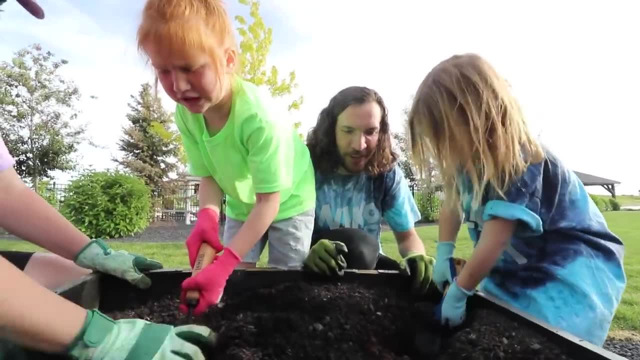 spots. so one right there and one right here. Yeah, Niko, how's your hole going? Okay, that's good. Guys, Niko dug a really big hole. That's perfect, That's good. Yeah, Oh, that's. 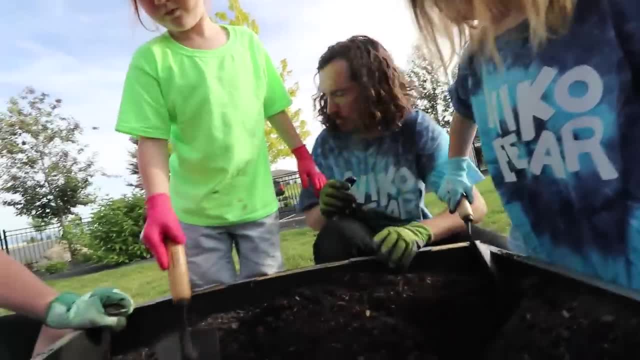 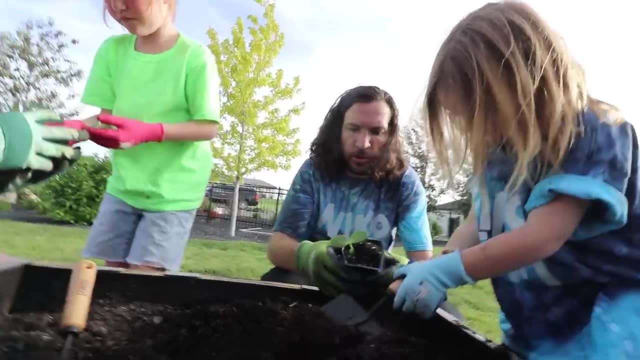 good, Are you a pirate boy? Yeah, Okay, Adley, grab the plant. I'm gonna teach you a trick: how to get it out. You gotta squeeze the black plastic around it, Squeeze, Squeeze, And then you're gonna go. 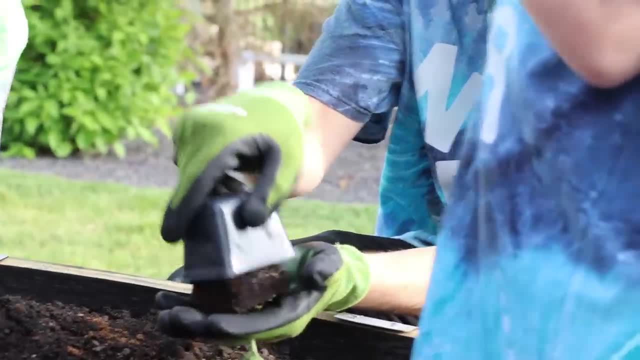 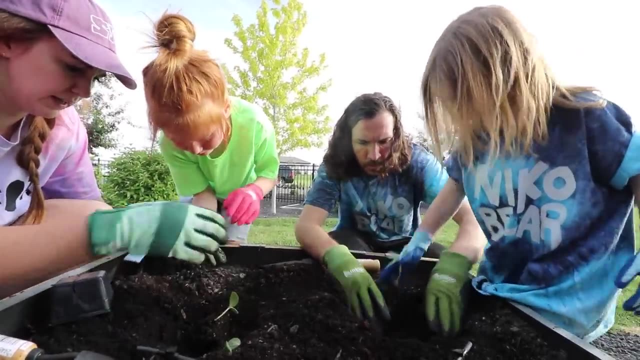 Can you do that? Uh-huh, Put your hand right here. Okay, we got the plant. Plant it in. Good job. There's a little seed. Okay, Right here. Good job. Oh yeah, Let's put that in there. You put the. 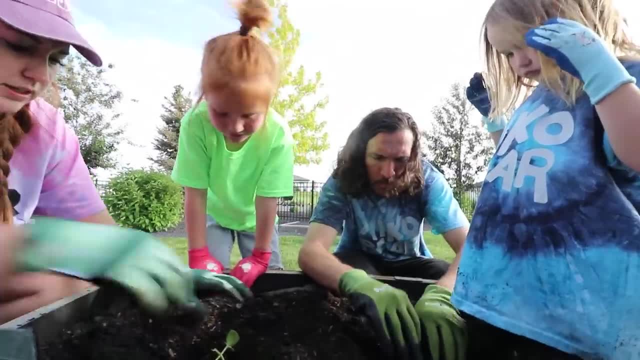 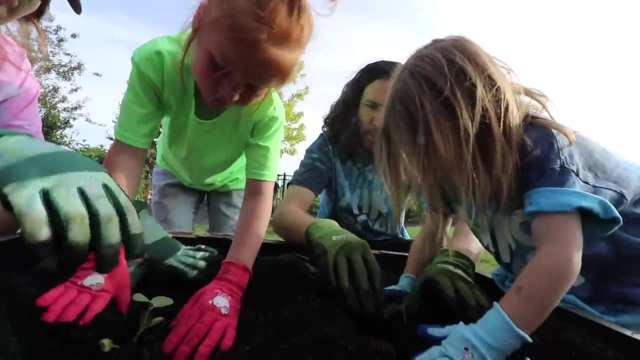 root back in. Niko says big, no, fair. Okay, and then we're gonna gently take the dirt and just pack it around. Okay, Scoop the dirt back in and make sure the leaves are up. Oh, good job, Niko. 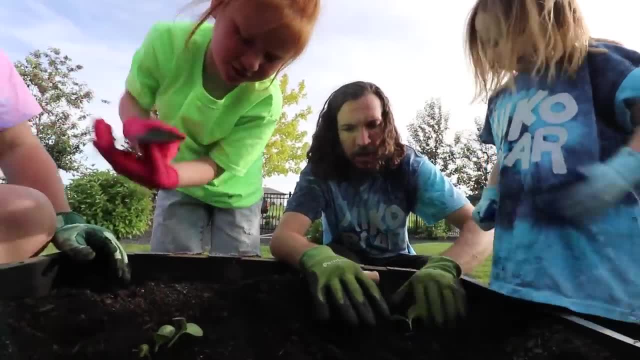 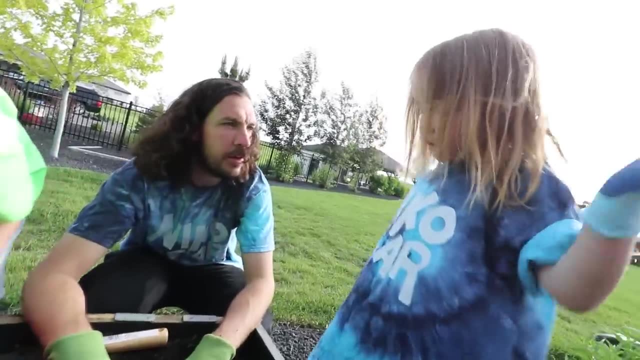 Okay, that's perfect amount. Wait, hold on, We got one more thing to do. Good job, Niko. look at your little watermelon plant. Oh, it looks perfect. Oh, this is water. Water, need water. They do need water, You're so. 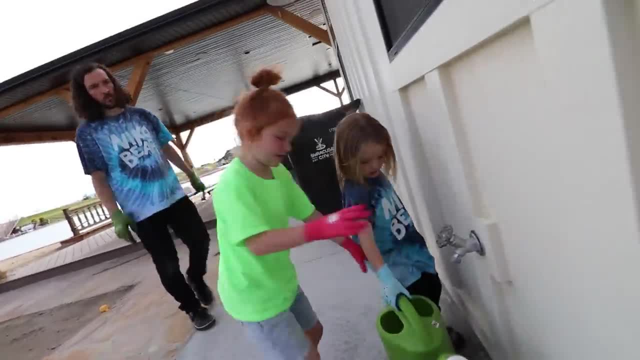 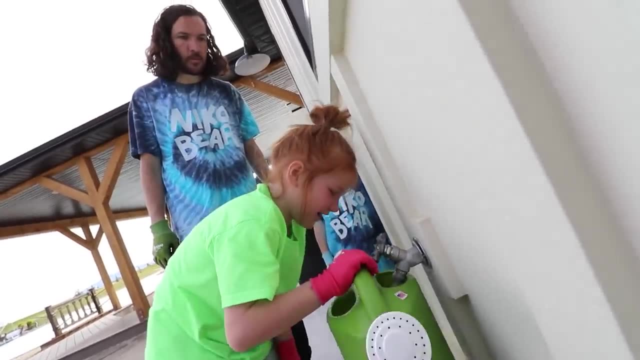 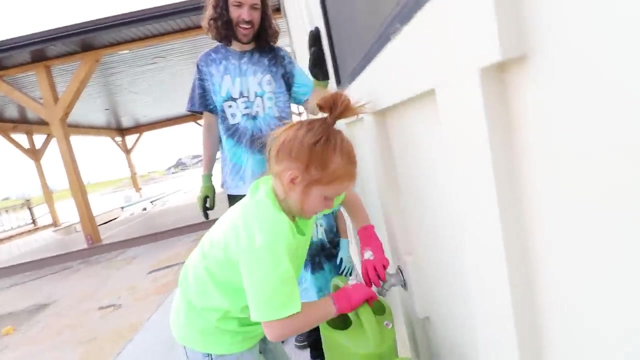 smart. There's the water. I know I can help you, Niko, You gotta hold it up. Good job. Okay, that's good. Okay, that's good. Not enough, Nope, not enough. That's not good, but it's not. 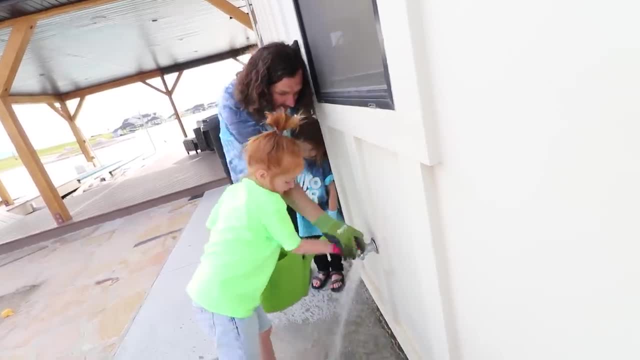 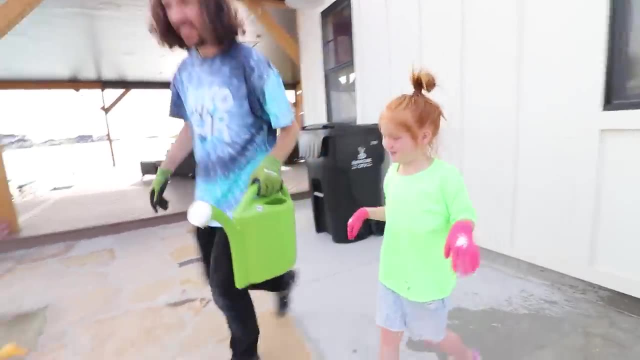 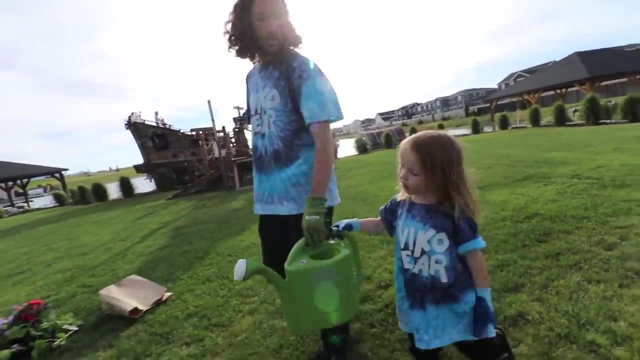 Okay, it's good. Wrong way, You're crazy. All right, let's go water some plants. You need some teamwork, Mom. my shoes are wet now. Dad, how do flowers drink the water? They drink it with. you know their roots. 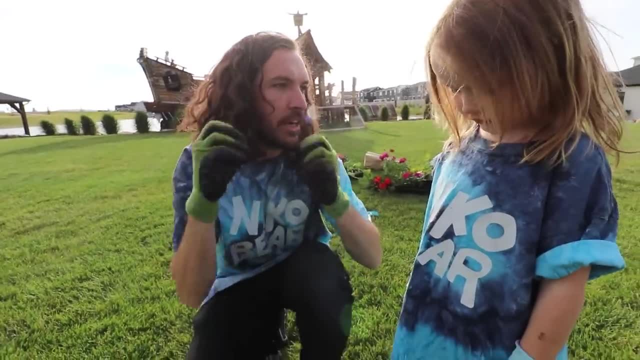 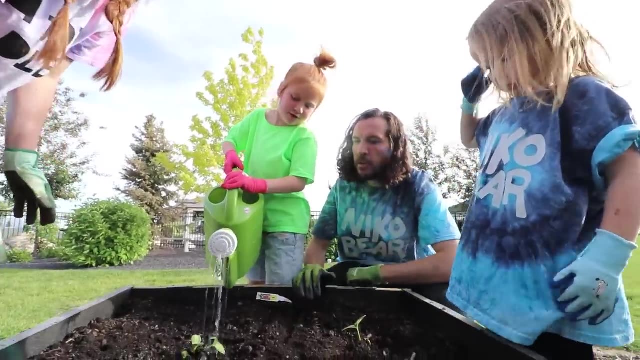 on the very bottom. Yeah, The water gets in the dirt and then the roots drink it up. They drink with their roots. Oh, I'll go do my first. Daddy, Me and Niko were just talking about how plants drink through their roots. Niko, do you want to help me? 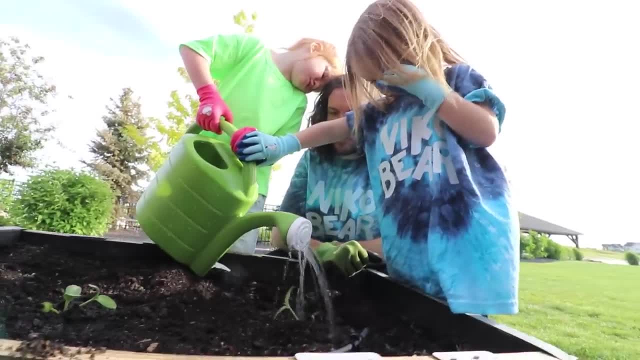 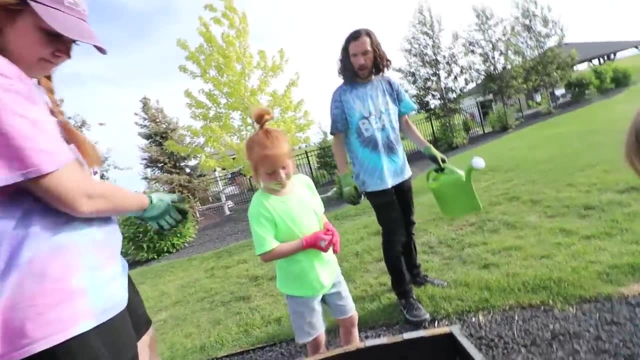 We gotta make sure we get it all the way down to the roots. Okay, that's good, And mine needs a little bit more. Okay, perfect, You can check on it right before we leave. All right, what's next? Next is pumpkins- Pumpkins. 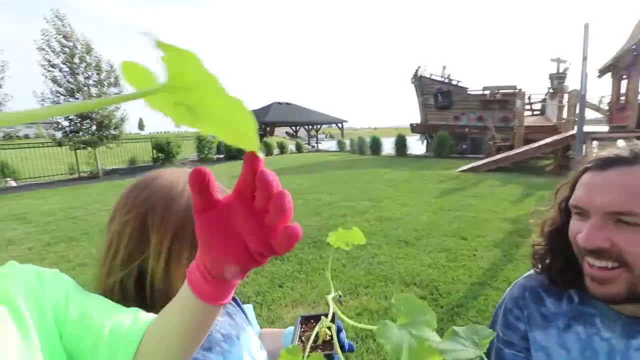 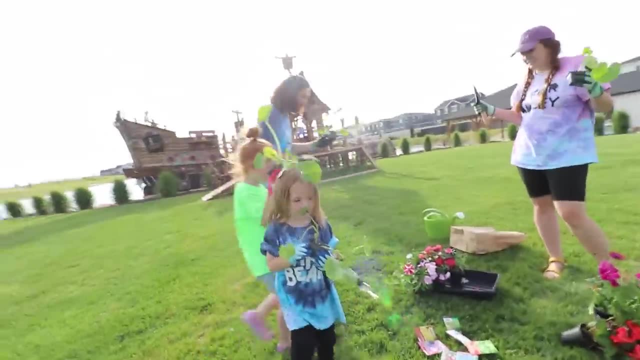 Pumpkins. We have four pumpkins. I've got two. Oh, Niko has two. It's tickling me. It's tickling me, No, tickling Adley, It's attacking. All right, grab your shovel. Water, Dad, Water. 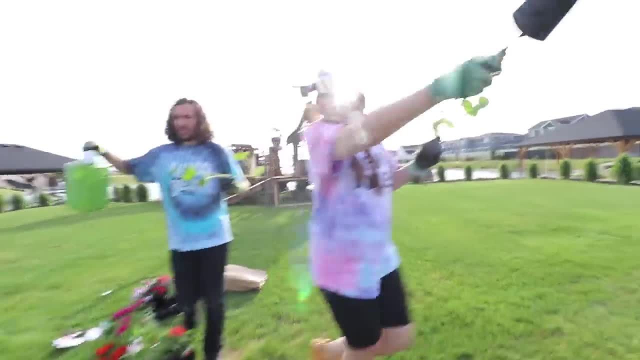 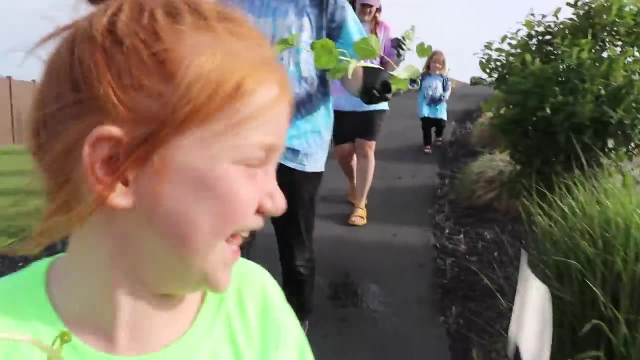 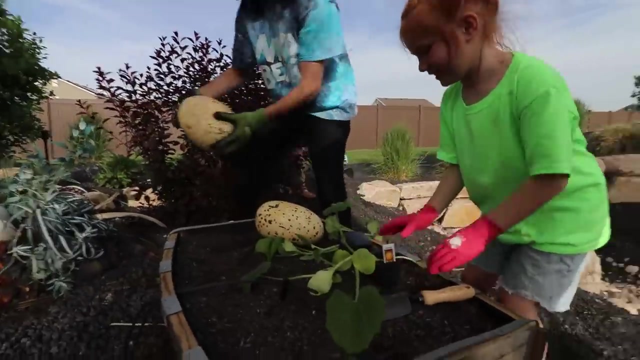 Okay, the pumpkins are over here by the mama dinosaur. Wait, does anyone feel like it's raining? It's not raining, I think it is. Hey, there's eggs in it. Eggs. Hey, we're not planting any eggs. Get in your nest. 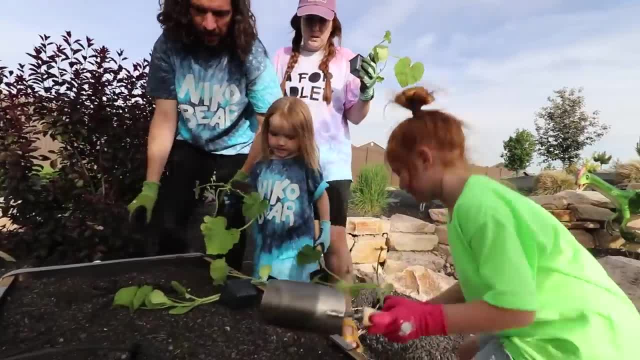 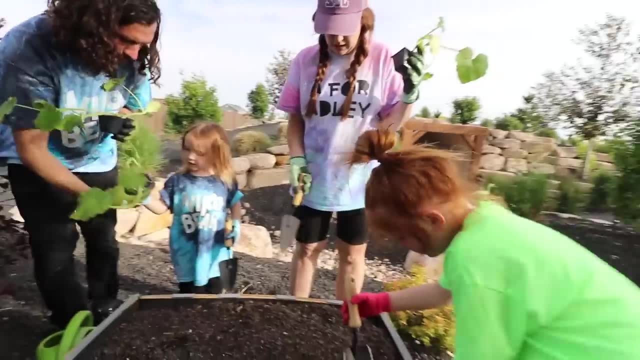 Okay, first we gotta dig holes. Okay, How many plants do we have? Four, One, two, three, four, So we'll probably do one in each corner. Dad, can you hold mine? Okay, I've got one right here. 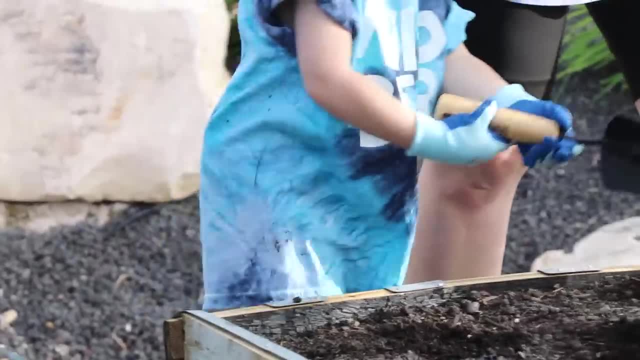 Okay, I've got one right here. This is mine. Oh, that looks good. I know what to do when I'm done: Squeeze, squeeze, Squeeze, squeeze, squeeze Upside down. Okay, you want to put it in? Yeah, Squeeze, squeeze. 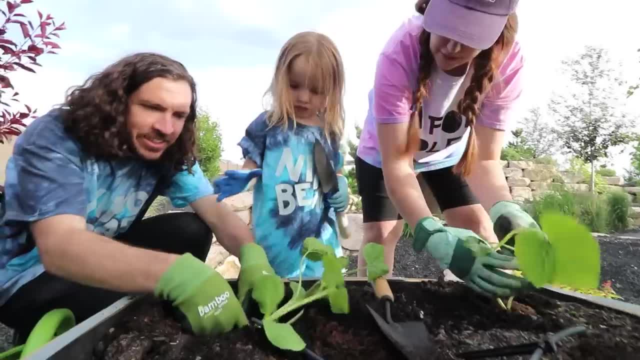 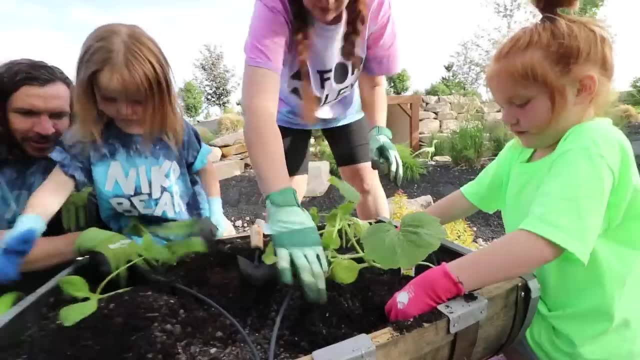 Put it inside there. Oh wow, Oh yeah. Good job With the leaves up, With the leaves up. Oh, I need a bigger hole. Good job, Niko. Mom, can you take it out and hold it? 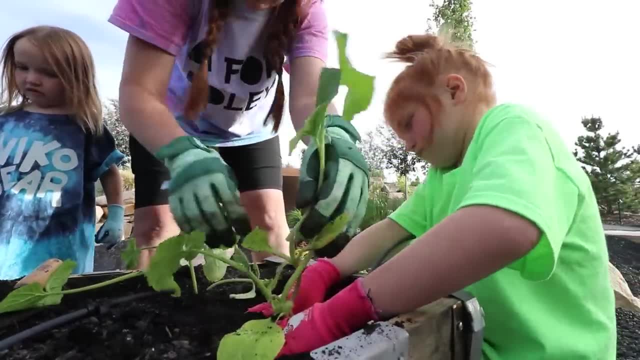 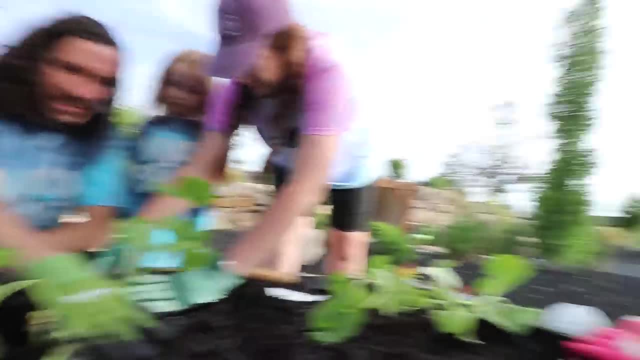 Sometimes it's good to hop on Yep, and then you gotta pat it down. Oh, I see a worm. Good job, Good job, buddy. Now we need to water it. I just had the water right here. Where did it go? 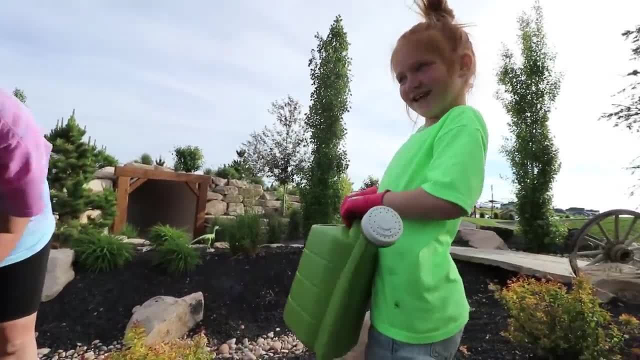 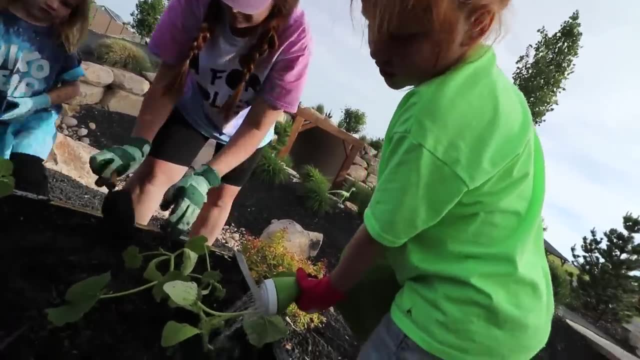 There's a water thief, the dinosaurs Who did it? Seriously, It was you, Adley. Hey, I'm gonna water me and mom. Okay, Mine needs lots because it's big, Mom's needs lots because it needs. 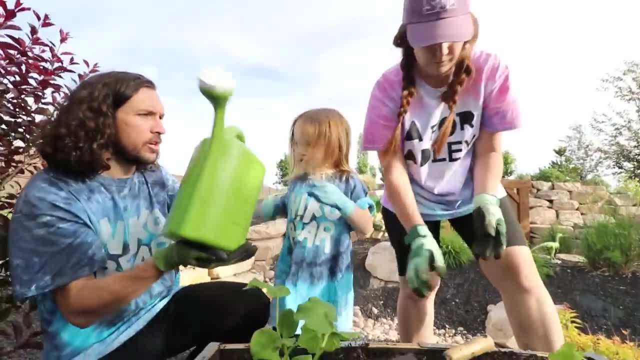 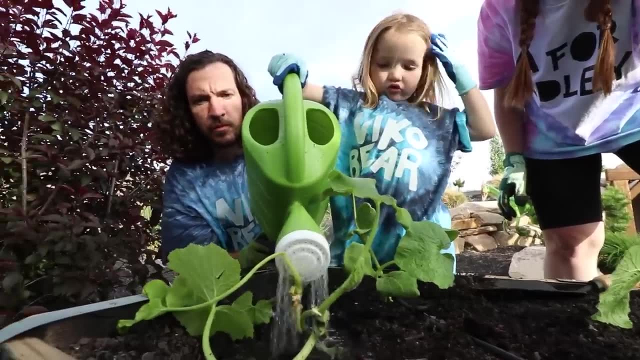 to grow nice and big. Niko, here you go. Okay, Niko, you ready, We need a lot. Yeah, do a lot. Oh, good job. Wow, that looks good. All right, I made the parasol water go through here. 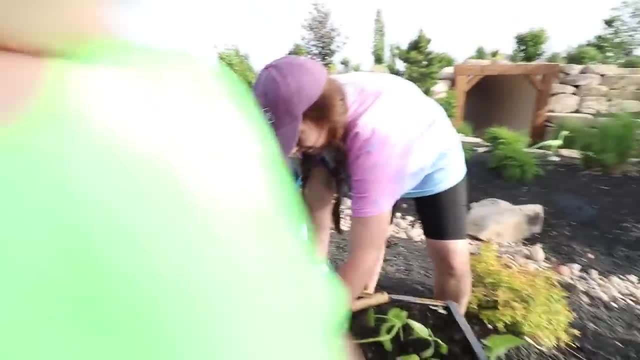 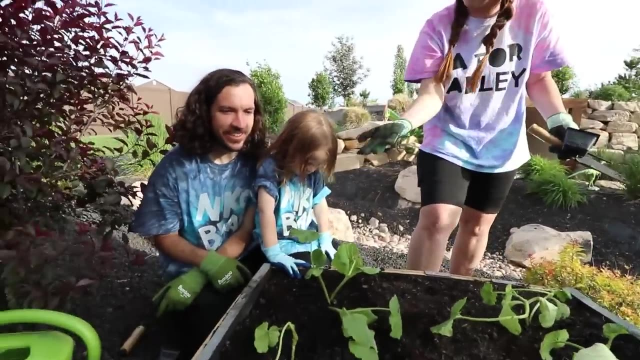 and to the other one. That's a good idea. Yeah, All right. what's next? I think flowers, Flowers. Should we go do the flowers? Do you guys have your plastic? Okay, Shovels water. Wait, Niko, is it raining? 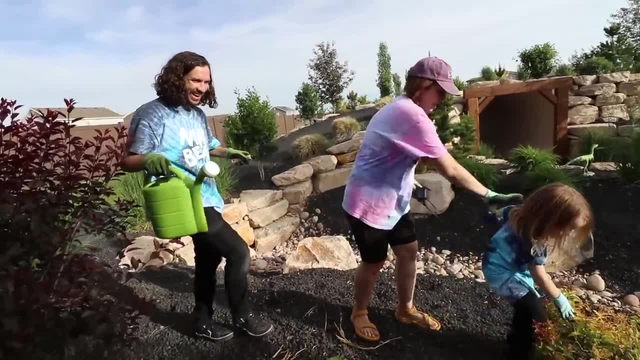 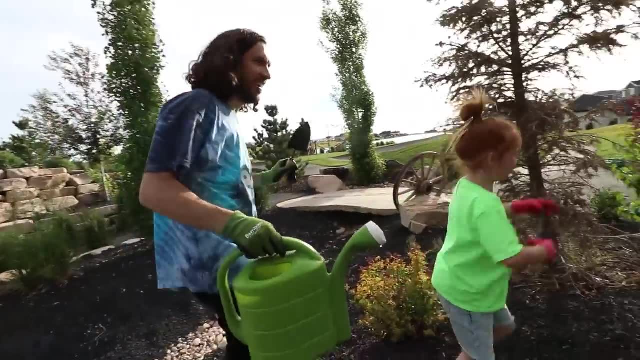 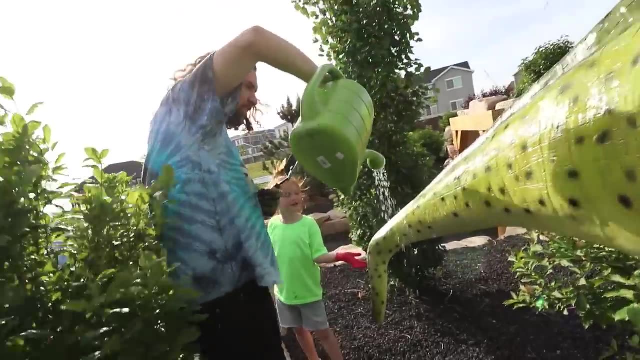 It's raining Vlog. is it raining, Dad? you're gonna waste our water. Okay, okay, I'm sorry. Big mama's hot There you go. Little bit of a shower for you. There's no more water. Oh, she's loving that. 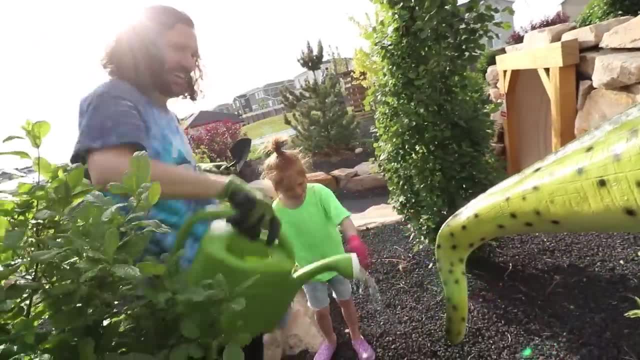 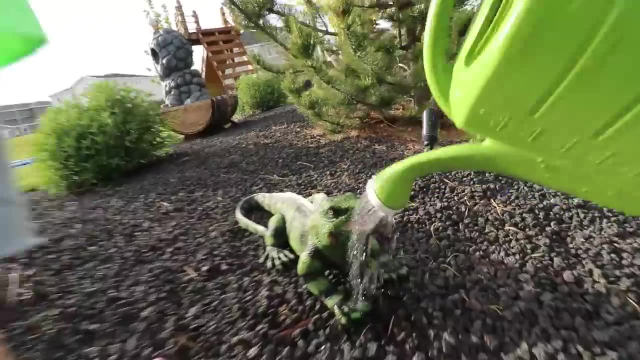 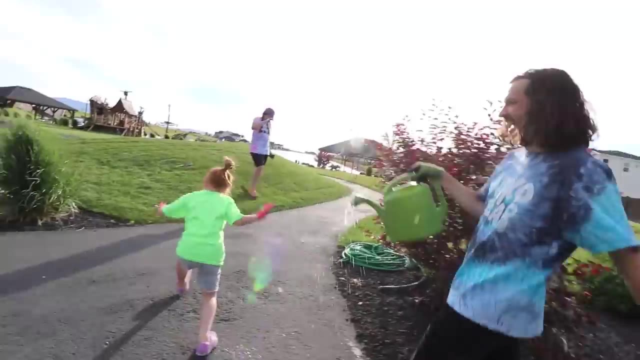 We can get more. Oh, she's loving that, Dad. I think the iguana needs a drink. You need a drink, buddy. Here you go. Mmm, delicious, Just a little drink, All right, what's next? 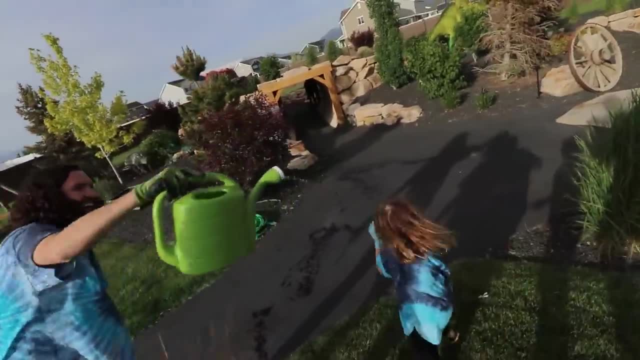 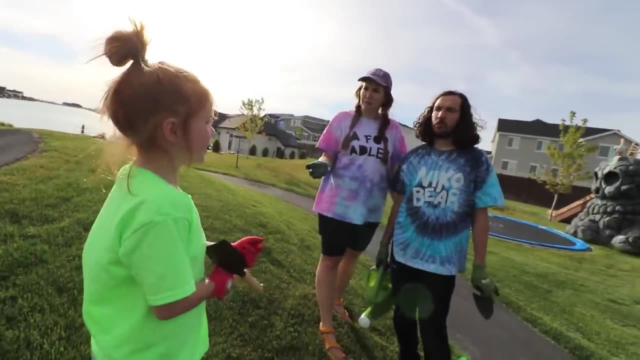 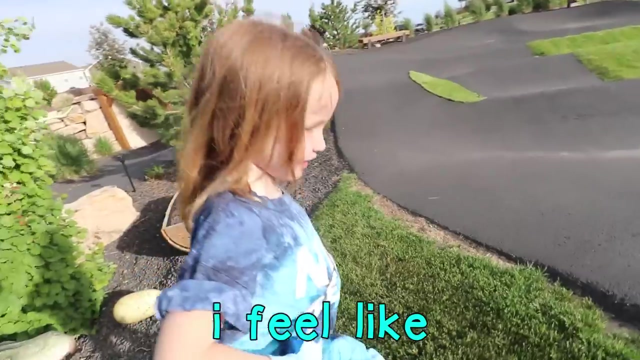 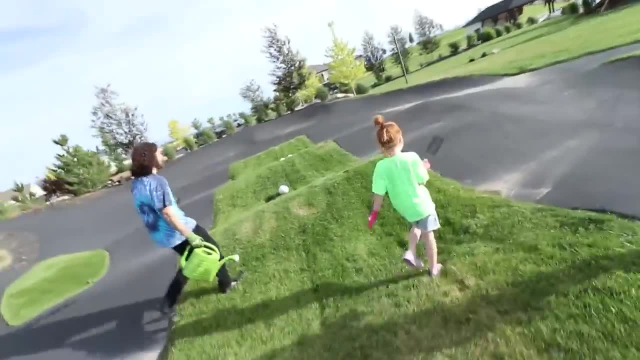 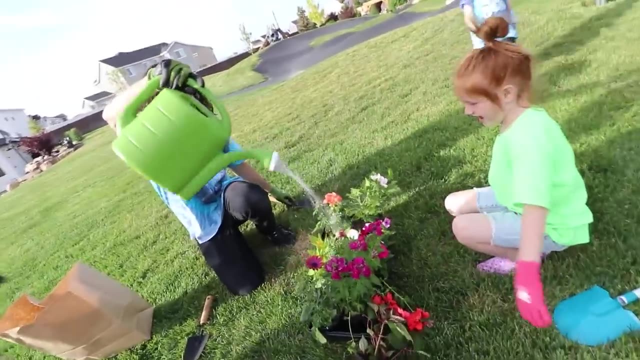 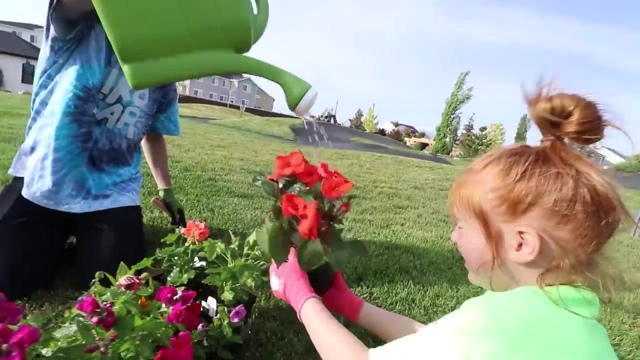 Oh, I better water you, so you grow. Water all the flowers. I bet we could fit all the flowers in one planter and then we could pick a vegetable or something to do in the other one. This flower's poor, This flower's poor. 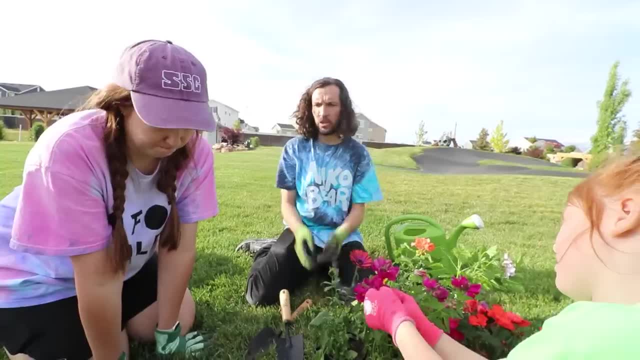 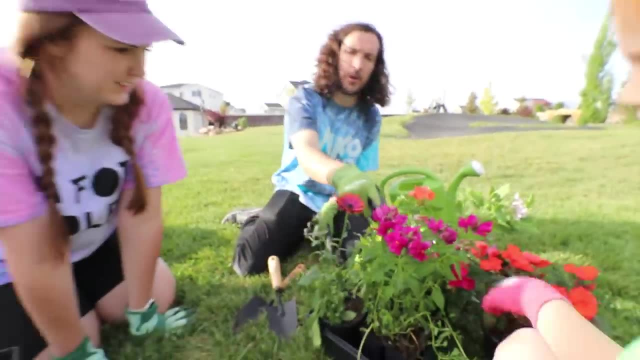 Okay, Dad, we water after we plant them. I know they just look so thirsty. So do we do flowers next or the seeds Flowers next. I'm bored of waiting. Those flowers are bored of waiting. Let's plant those next. I'll carry them over. 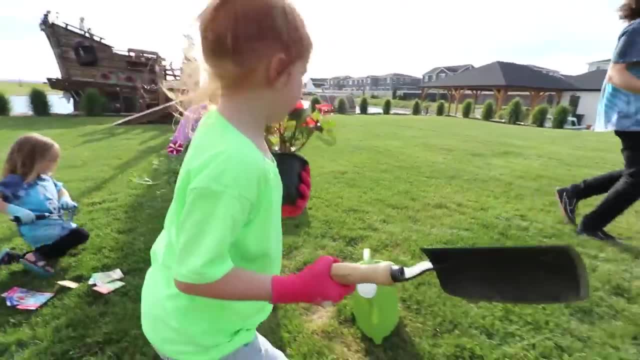 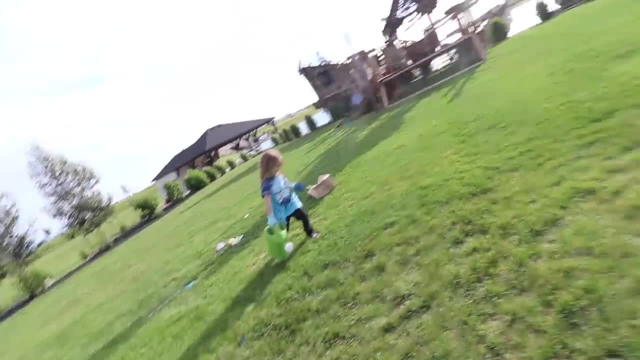 Grab the flowers, Shovels And the water. Grab the water, Niko. Okay, I'll drop it. No, Niko, No, Here, vloggy, I'll dig you up right here and you can have your own home. 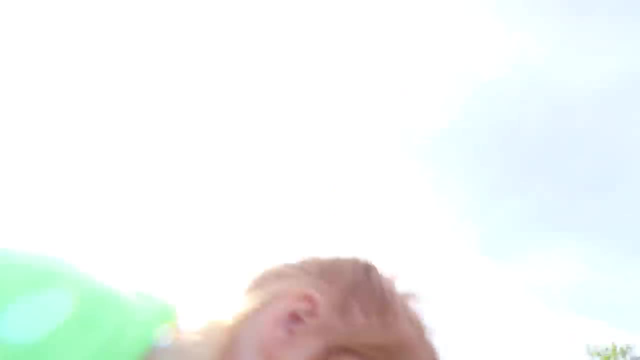 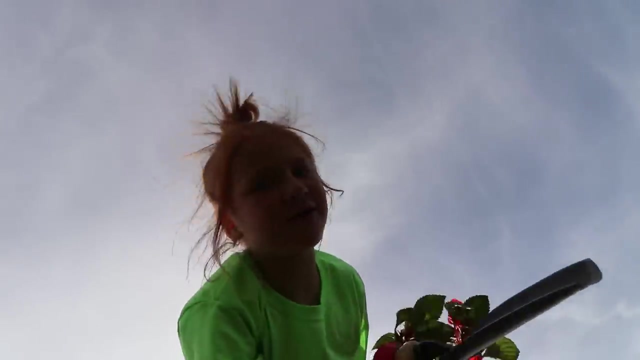 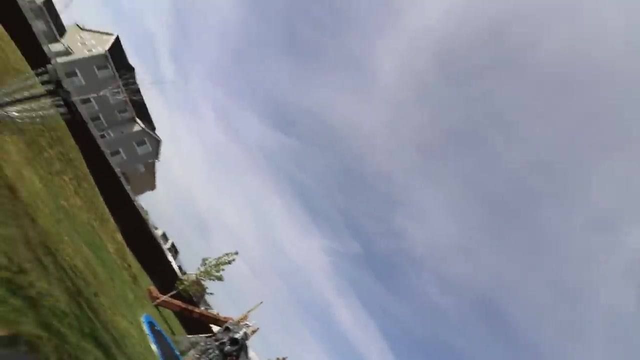 Dad, is this how you plant flowers? No, over here, Plant the vloggy, Don't plant the vlog. Don't worry, vlog, I would never really plant you. Oh, you're heavy. Come on A little cameraman. 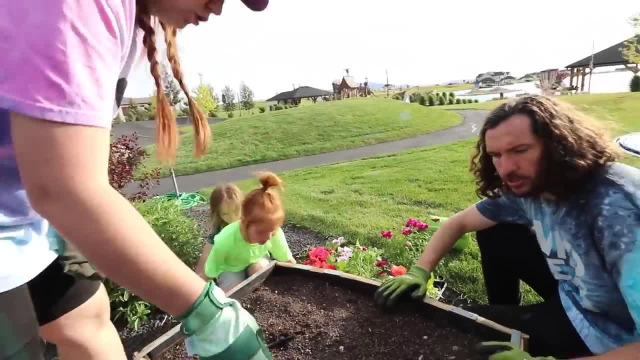 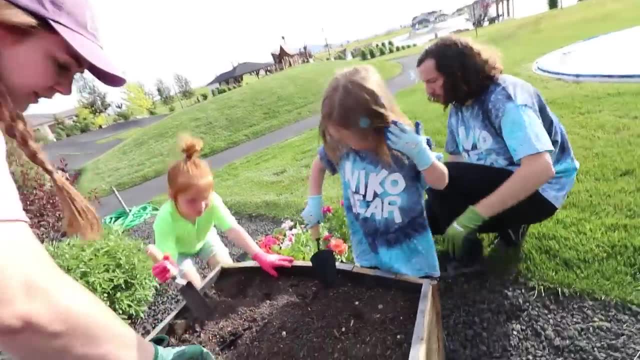 Alright, where's the shovels? Alright, let's dig some holes. We should do the tall ones in the back and then the shorter ones up front. Do you want to start digging some holes? bud, Start digging some holes. Oh, I'm going to dig one right here. 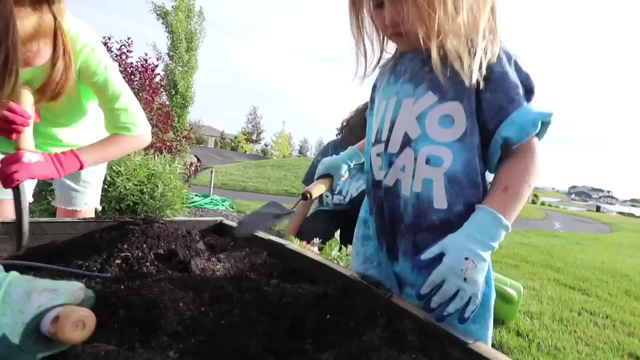 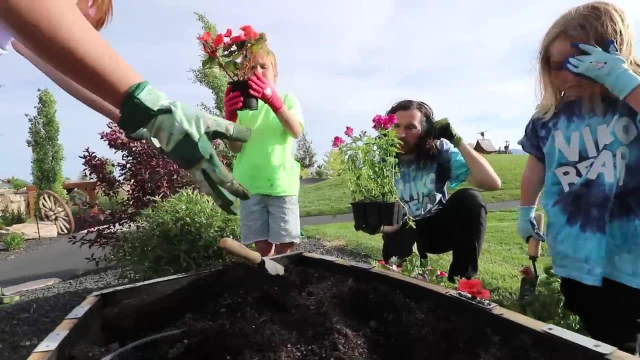 Oh, good job, I'm going to put one right on the edge right here. Oh, we should put the snapdragons in the back because they're tall. I want to put this one in the back. Oh, that's cute. 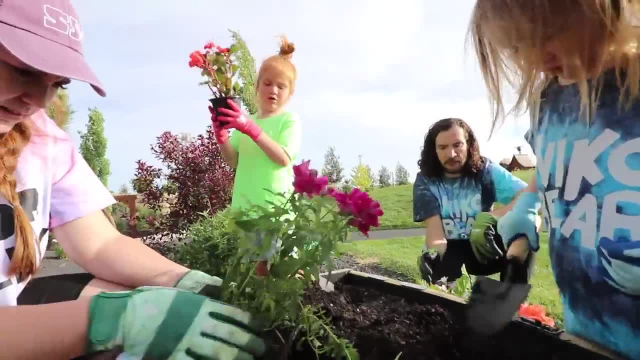 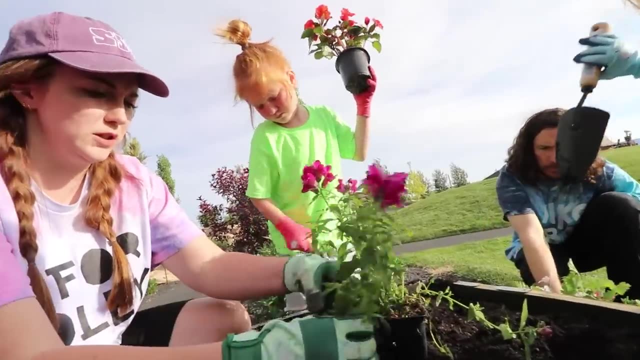 How many are tall? Tall, Alright. Oh wow, There's six. Oh, we can plant six of them. Hold up the leaves. Who wants to scoop the dirt around it? Holy cow, Whoa Adley, That's a big one. 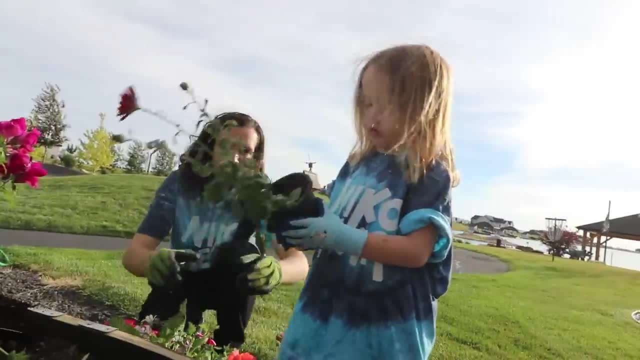 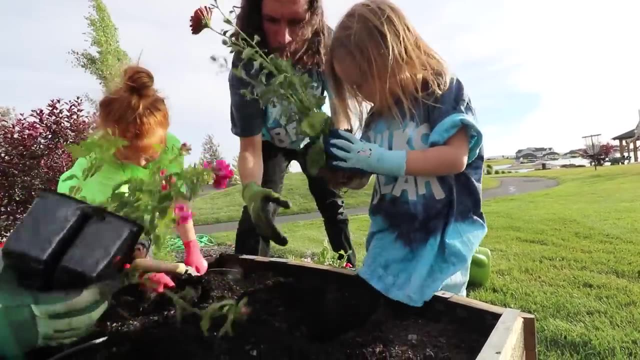 Oh, it's humongous, That's a good spot. Oh, plant it back here, bud. Flip it around, Alright, And then put it in the dirt. Find a good hole. This is my hole. Oh, right there. 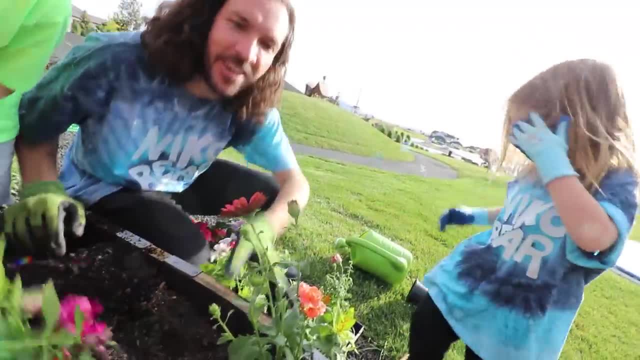 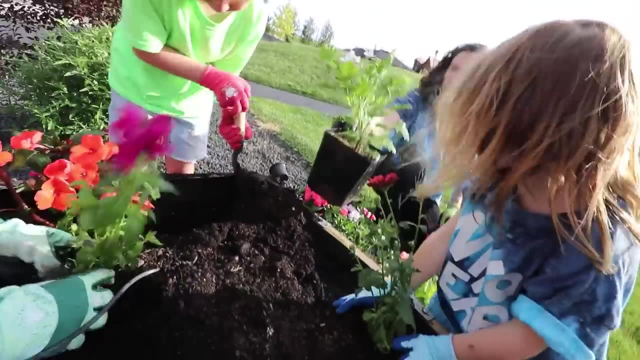 Oh, that's a good spot. Does it smell good? No, I'm digging here, Sorry. Oh, here's a big one. This one probably needs to go in the back. It's pretty big. I'm already planting something. 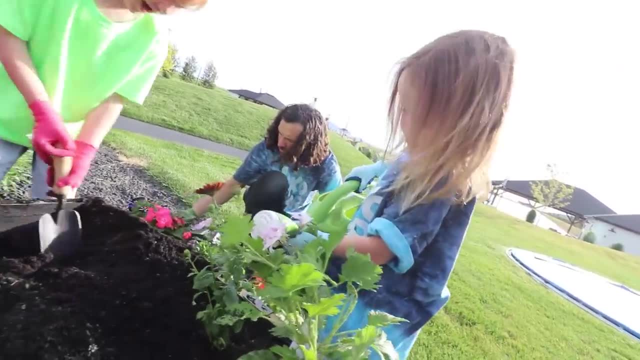 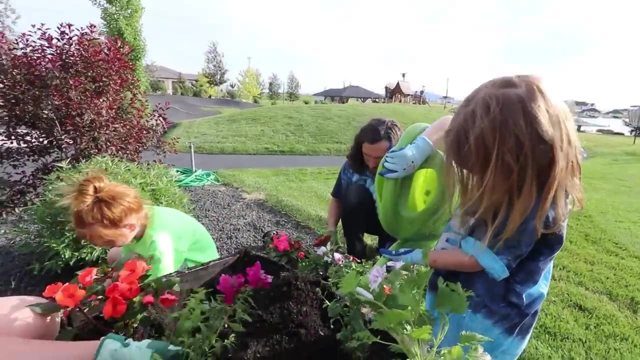 Okay, Hey, watch where you're throwing some dirt here. I'm sorry, I have to make a big spot for these guys. They're pretty big, Pretty big. I think the fairies are going to like these flowers. Yeah, Wait, Mom, Where are the fairies? 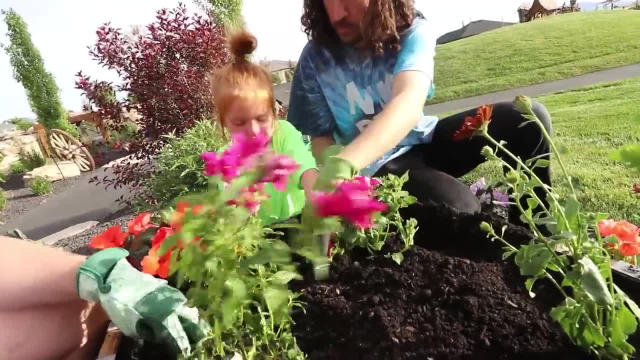 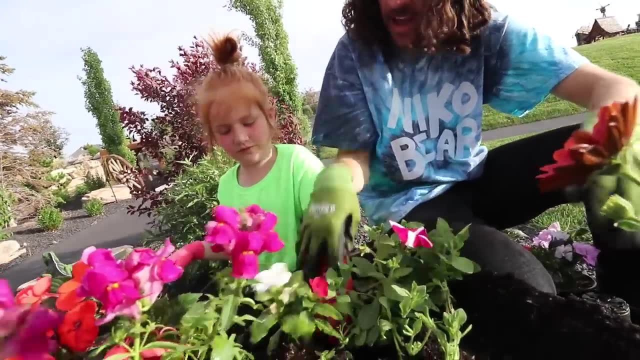 Oh yeah, I like these flowers, I like them too. Oh sorry, We can be neighbors. Hi neighbor, That just means they're friends, They're holding hands, Little leaf hands, Yeah, but I still have more than that. 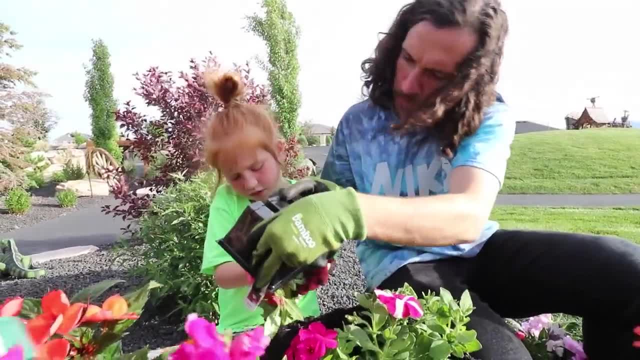 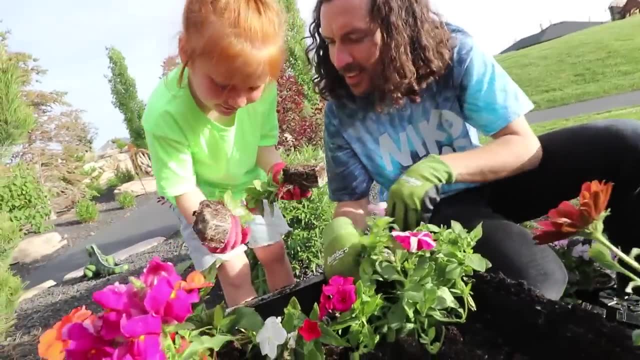 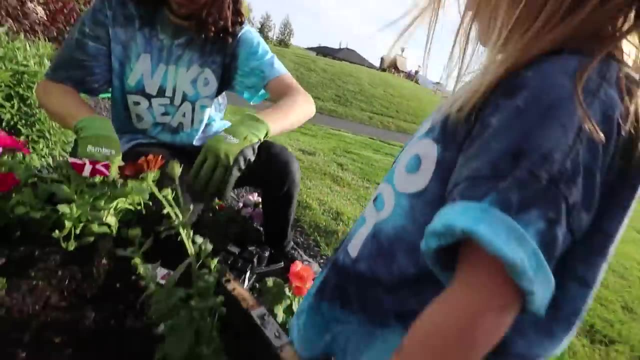 Okay, here I'll give you more space. They're excited to go to their new home. Hey, they were friends. Hey, you're pointing a tag. Alright, Is everyone ready in their new houses? This guy's ready for his new house. 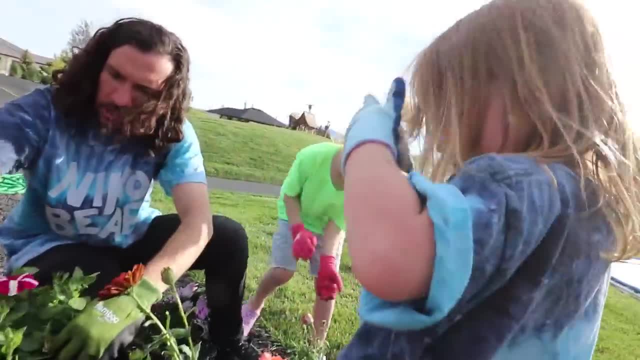 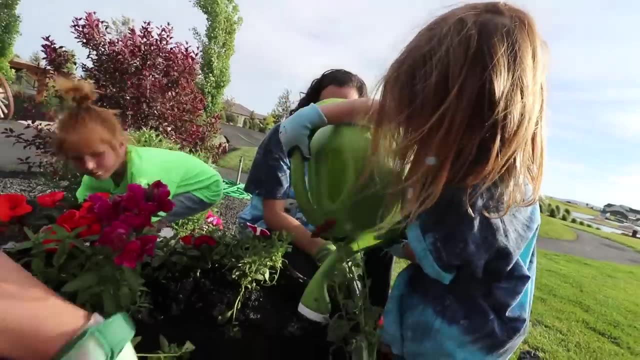 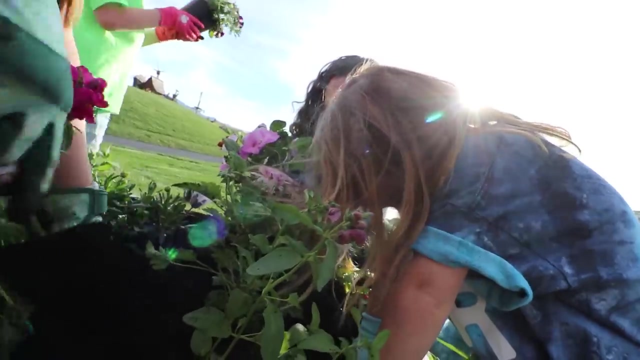 Niko, can we get some water on these new flowers? This one's really nice Get some water in the window. Oh yeah, This is a mosquito plant. I hope it works. No mosquitoes by our fairy forest, Ready, Ready. 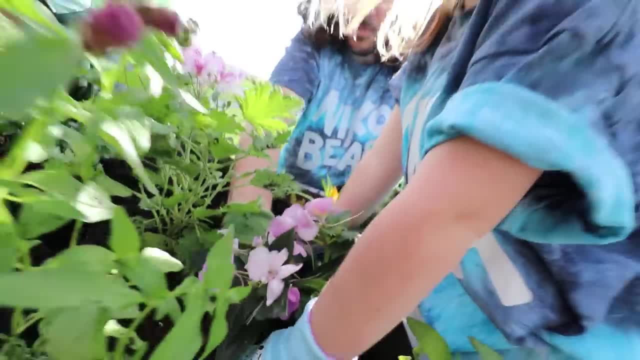 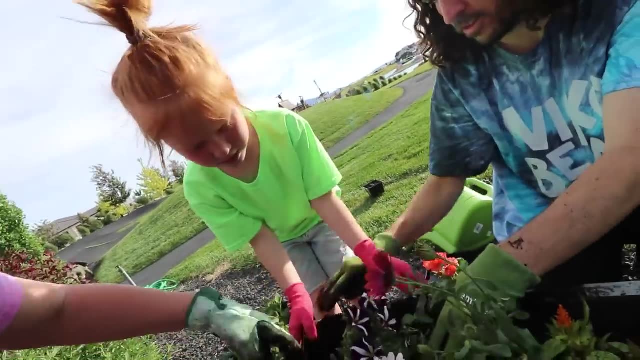 Alright, Put the dirt on, There's a hole. Wait, you should do that one up front. It's little Alright, That's a good spot for that guy. There we go. Oh yeah, Check, check, check. 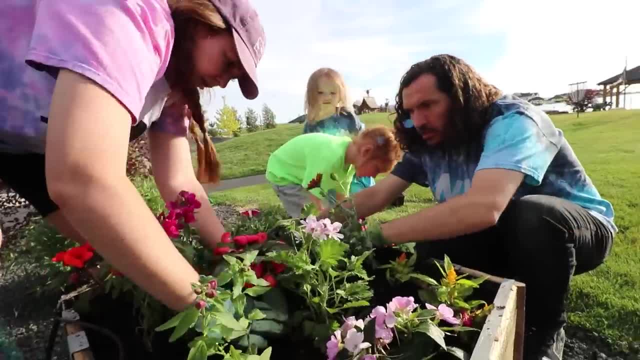 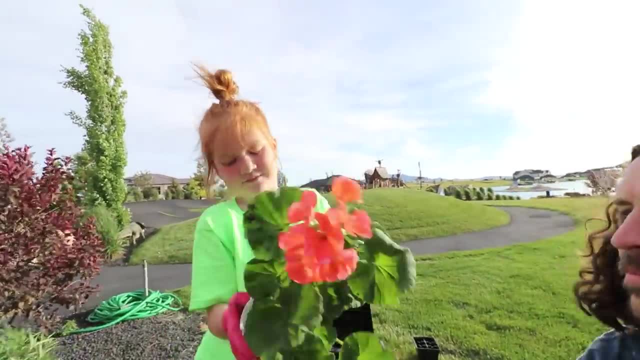 These flowers are going to love their new home on Pirate Island. I hope they're all really good friends. Oh, this one's wet. I wonder why they're wet? Because they're happy and healthy. So, Dad, will you hold the bottom. Okay, I can grab. 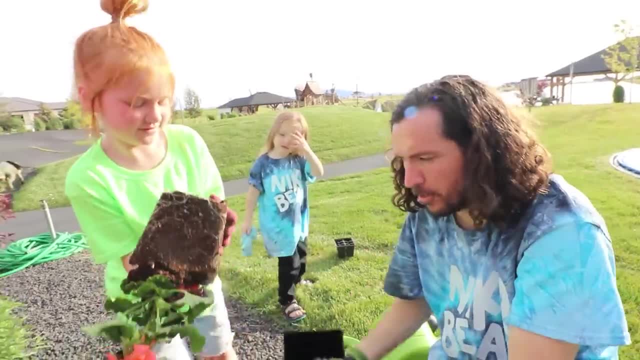 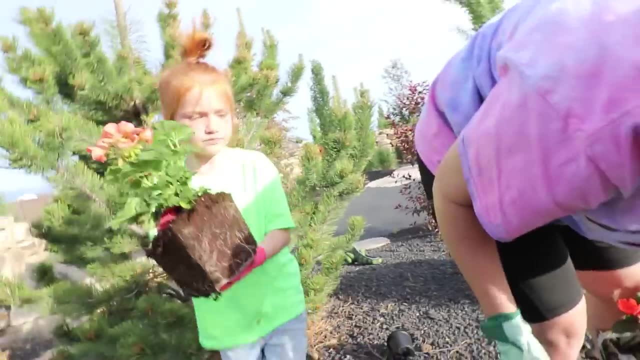 this one, Okay, ready, Oh, we got a big one. We got a big baby. Where are we putting this big one? There's one right here. Is that the spot? Move these guys over a little Right there, Oh yeah. 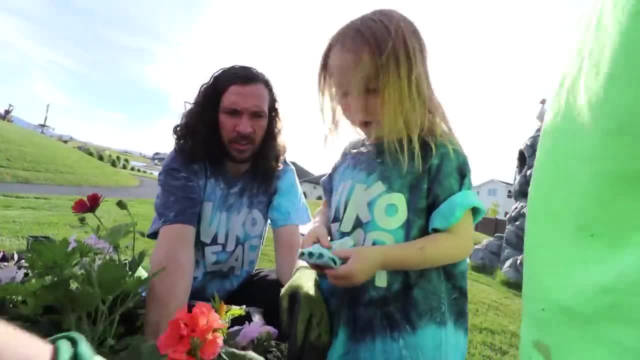 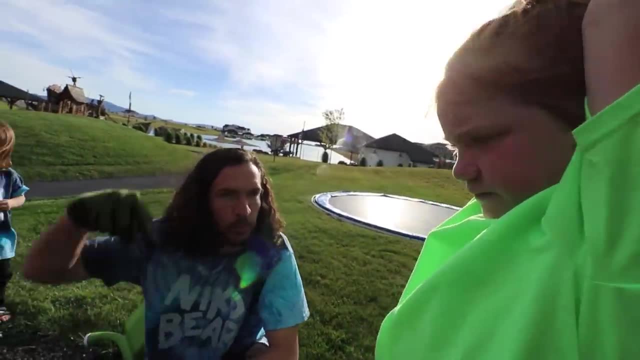 Oh, my hands are gone. Now I look big. I think we're ready to plant some seeds. Oh, the seeds are fun to plant because you have to poke holes. put a little seed in, give it some water, give it a little. 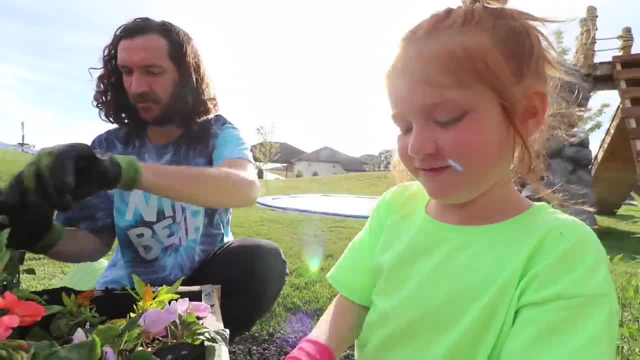 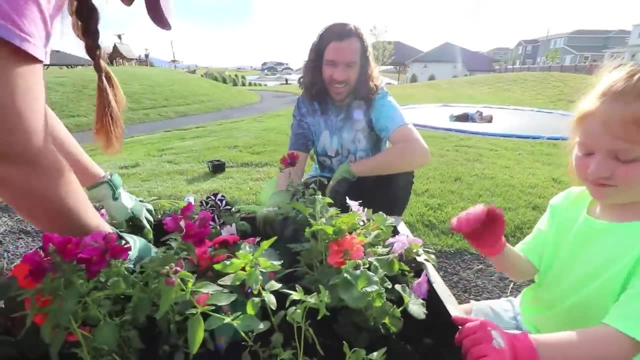 kiss. Good luck growing. Good luck growing. This looks good, So good. The fairies are going to love it. Wait me and Mom are the fairies. I love it, I love it, I love it. Even the pirates feel it. 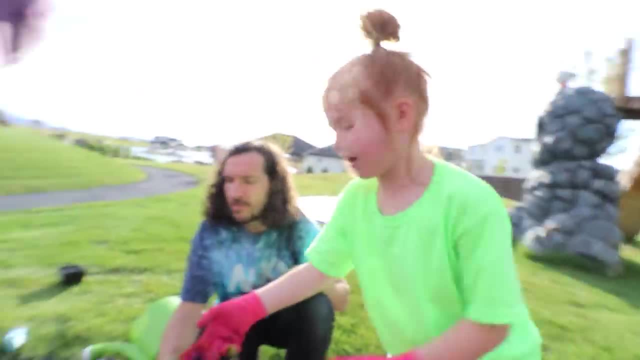 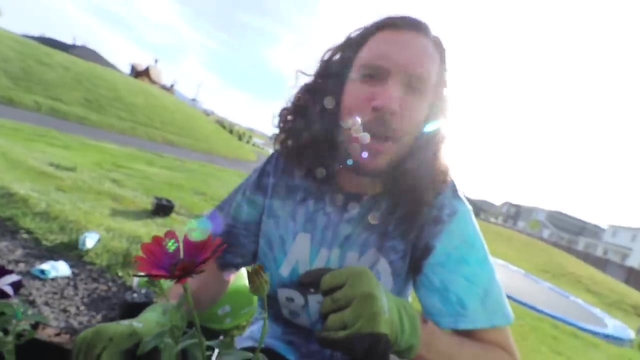 I'm loving it. Wait, can pirates love flowers? Oh yeah, Only brown ones like this one, Arr big man. Arr, Oh, so beautiful. Don't tell me other pirate friends but I love flowers, Dad. but 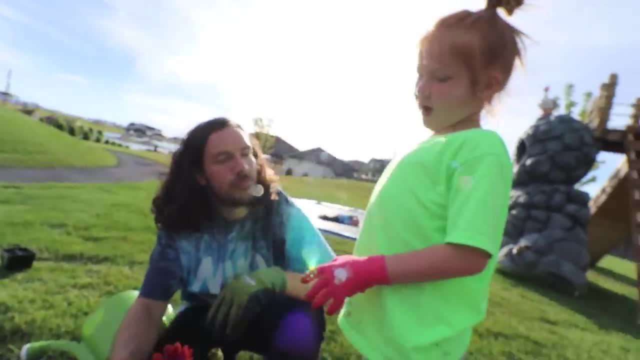 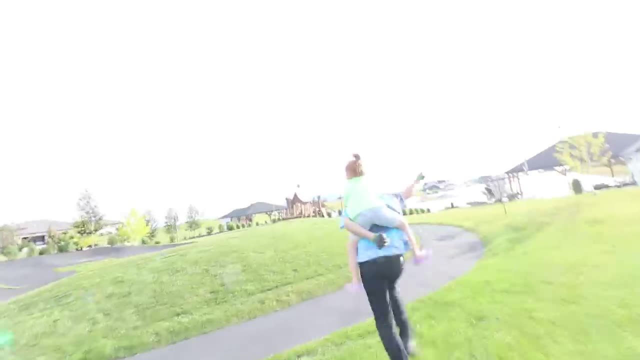 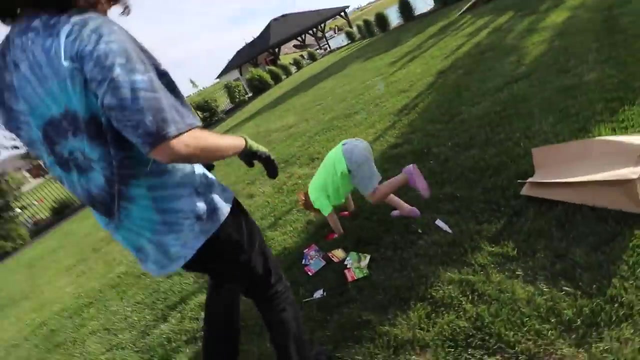 this, this, this flower smells like root beer bombs. Ah, root beer bomb. Let's go get the seeds. Seeds, Charge This beer, stop. Wait, we forgot to plant these flowers. Oh yeah, We can plant them with our vegetables. We got some flower. 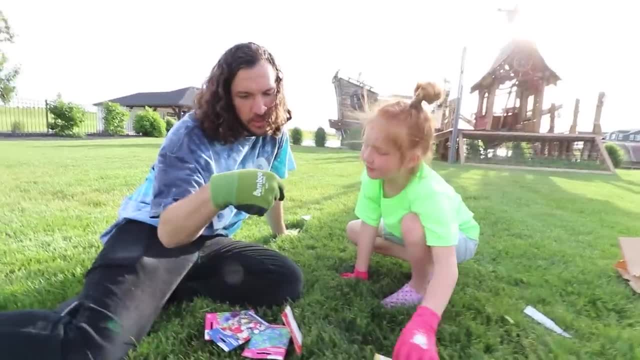 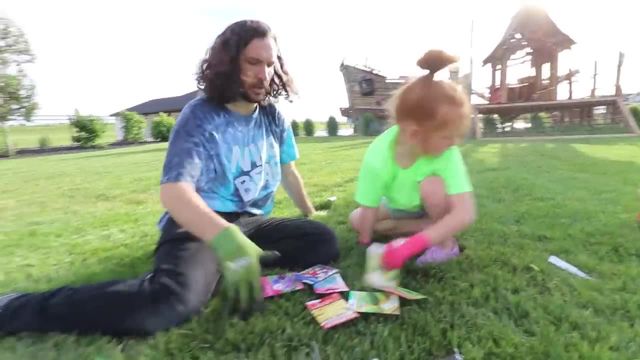 seeds. We got some corn. We got cucumbers, Some cucumbers, Two cucumbers And salad. Alright, We'll plant these seeds in another one. Should we go? Yep, let's go, Okay, Ah, Dad. 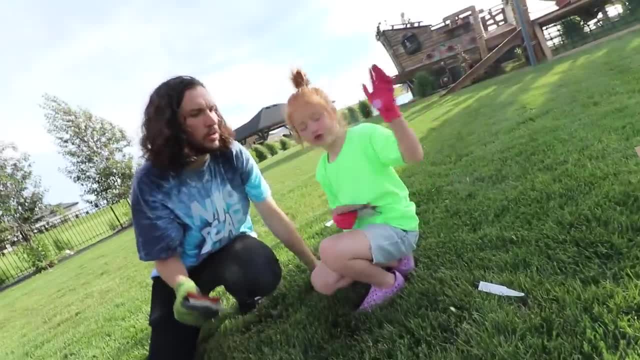 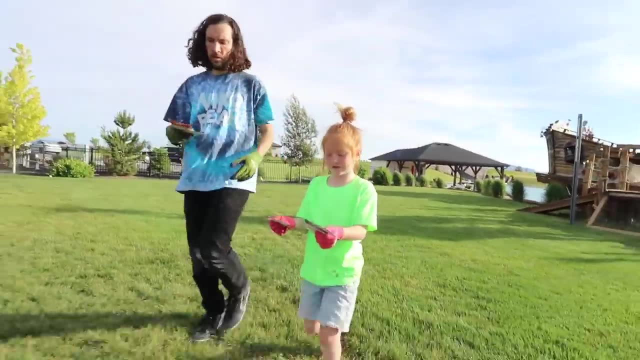 you're going to rip them, Alright. alright, Dad, we're not going to plant two cucumbers, We're going to leave those ones here, Deal? I only got flowers in my hand. Hey, I only got vegetables in my hand. How did? 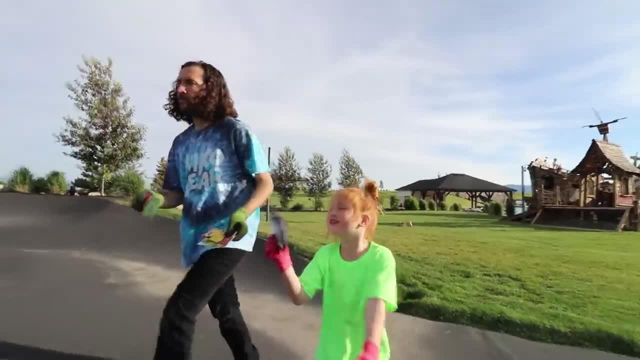 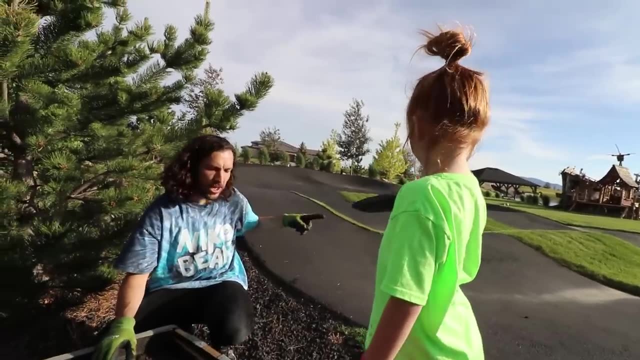 that work. I like flowers. You have vegetables. I like vegetables. I like flowers. I like cereal, I mean vegetables. This looks like a good place for seeds. I could be skateboarding on the pump track and then be like, hmm, I want some. 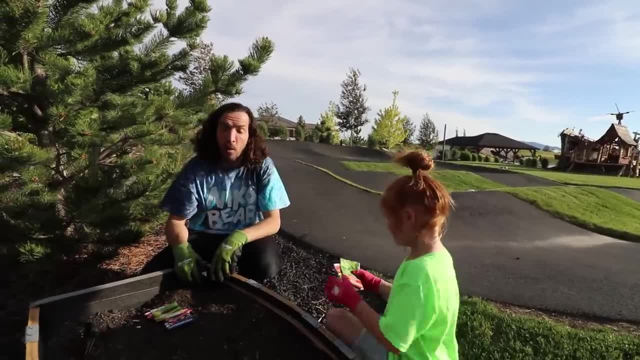 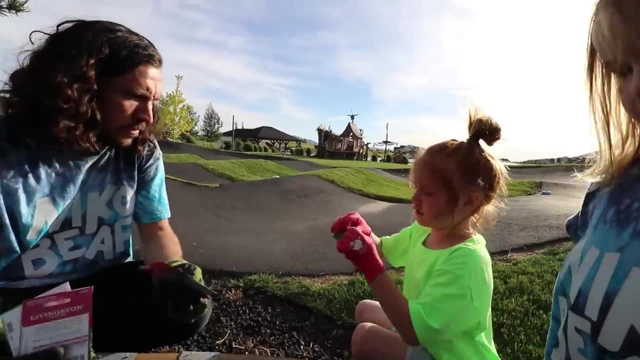 corn. Yeah, I know nothing about planting corn or if this is big enough, but we're going to find out. That's how you learn: It's by trial and error. Wait, look, look, look, There's a little sticky. 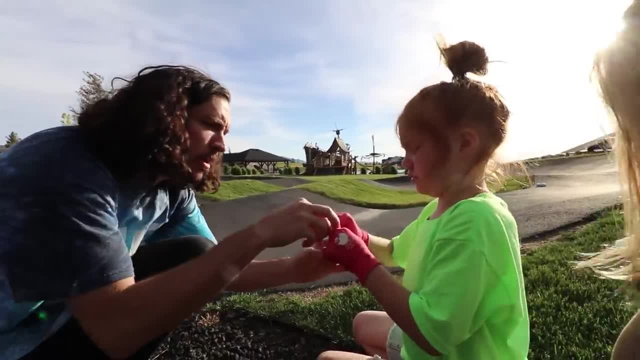 Oh, good job Here I can take my gloves off and help You do that. I'm going to start digging a hole for them. Oh yeah, we need holes. Wait, we got to read the instructions. I know nothing about. 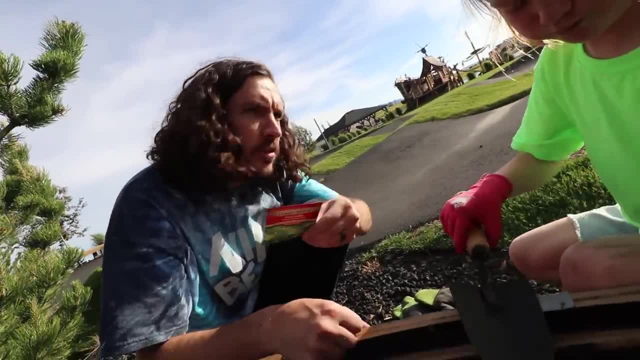 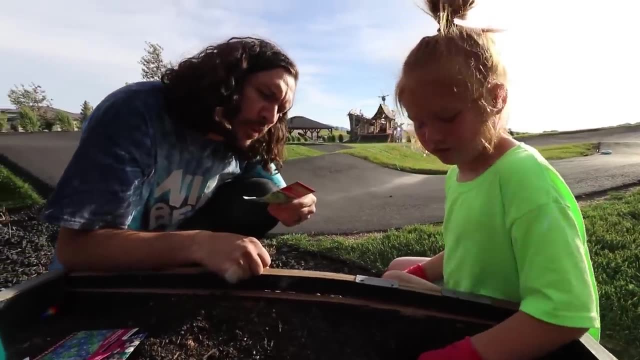 planting vegetables. Sow directly in the garden. Do you have a sowing machine? No, Why do we have to sow the garden? No, you have to do this. That's kind of like sowing. Okay, We'll see if we can grow some mustard. 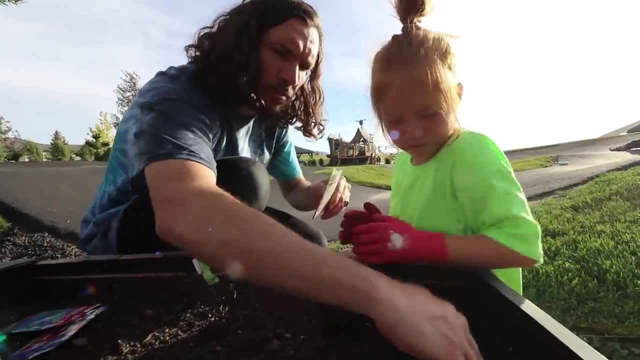 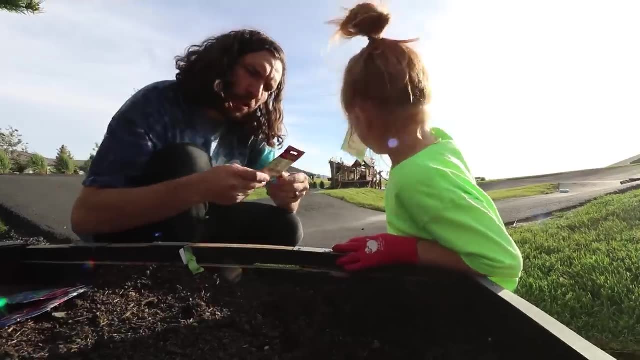 leaves, And maybe we'll put some over here too. Alright, Is there a bag right there? I think that works. We probably have mom here to supervise, but oh well, We're learning. Ooh, what do you think? corn? 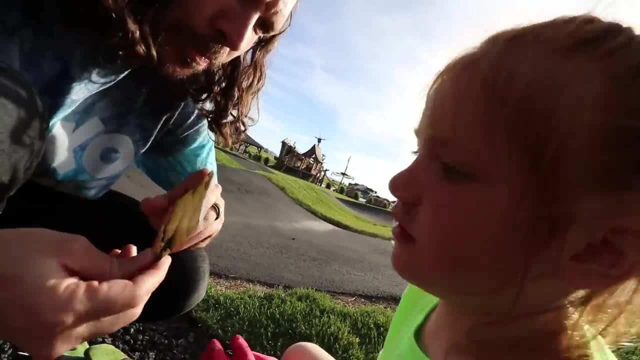 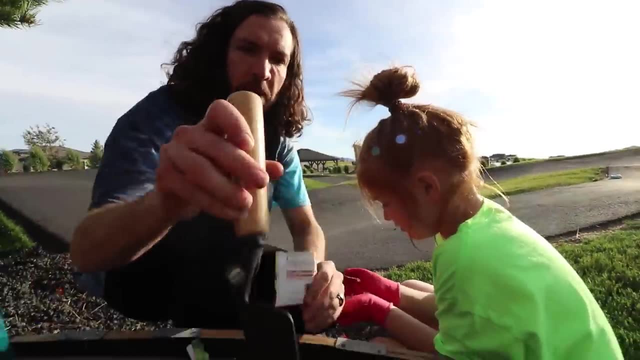 looks like. What do you think corn seeds look like? Oh, I knew it, It looks like corn. Oh, we need the holes. Okay, so back here, we'll do our corn. We'll put some right there, Dup, dup. 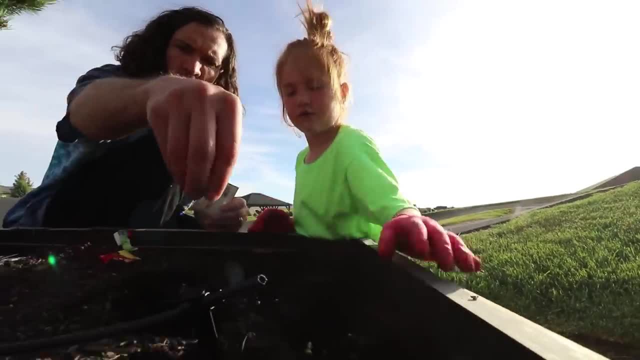 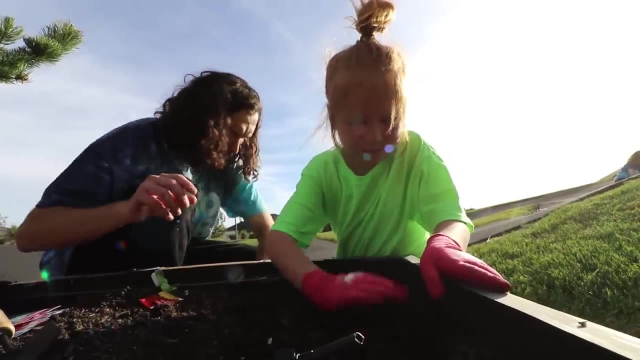 Dup, dup, dup. Those ones will go right there, Those ones will go right here, And then the rest of the pack will go right there. The rest of the pack will go right there. Now we cover it up. Oh, I forgot to read the instructions. 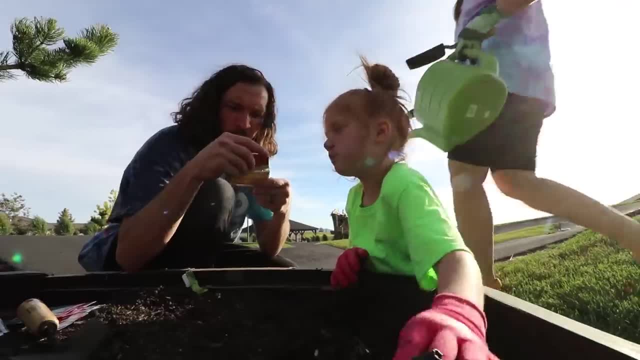 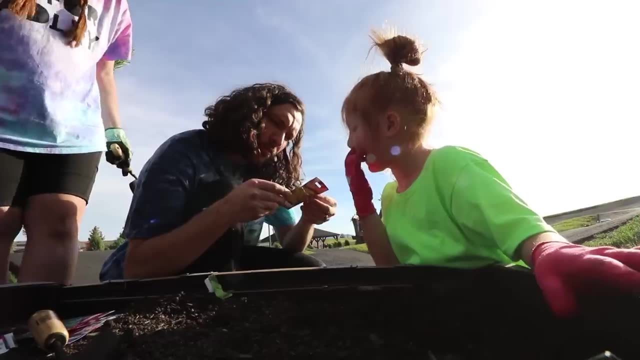 Oh no, I only have half the instructions. Okay, I got the water set up over there. What are we planting here? We need some mom supervision. We just planted some salad and some corn. Oh, really, Yeah, Okay, that's gonna be great. 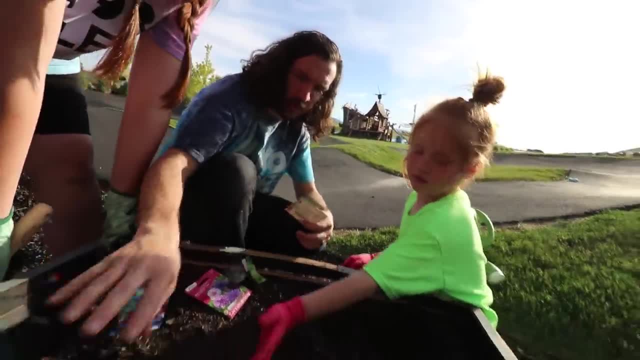 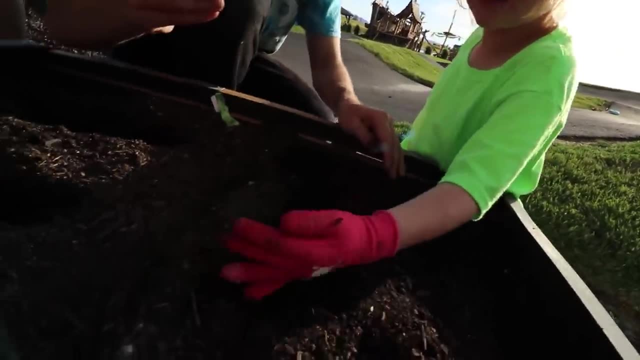 Should we do some cucumbers? We're kind of doing vegetables over here and then flowers over here. Okay, Is that your line? Yep, One, two, three, Oh, that's what they look like. There you go. I like cucumbers. They're yummy, I know. 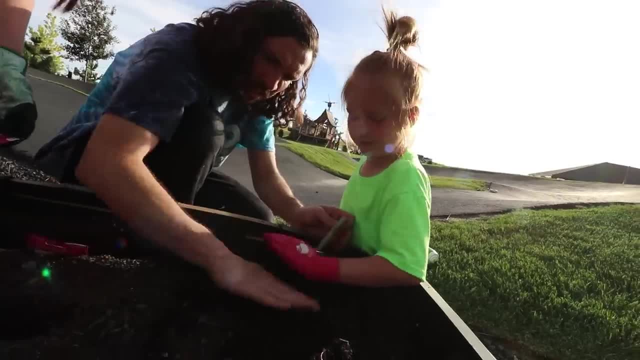 I like to put them on my eyes so I can relax. All right, tuck them in. Good night, kids. See you in the morning when we grow into a plant. Mom, what are you doing? I don't know. Is that how you do it? 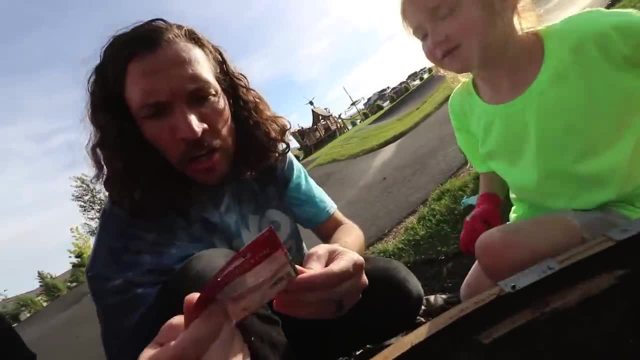 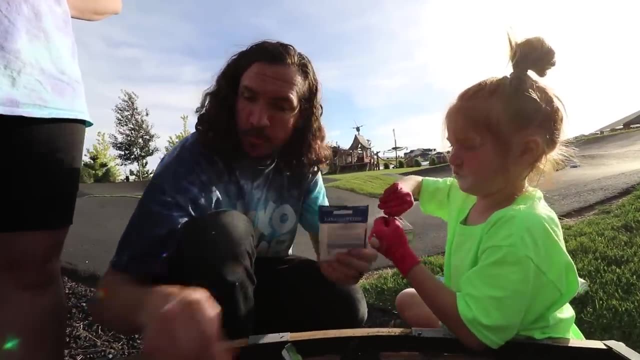 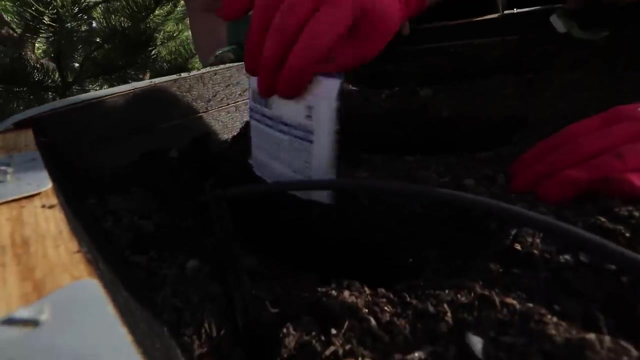 No, Mom, Okay, teach me. Okay, these are bachelor button flowers, Bachelor buttons, Yeah, Wow. And these are wild flower mixture. Ooh, pretty, And this is weather glass. All right, spread them out, Tuck them in. 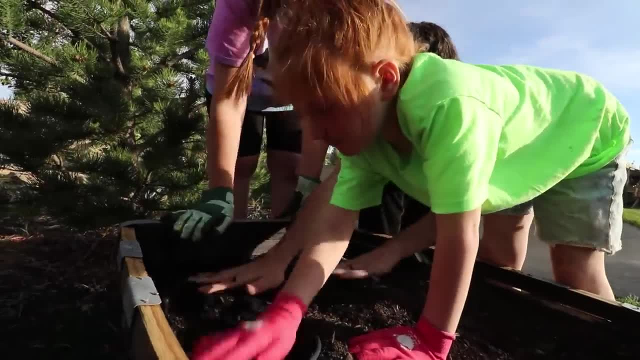 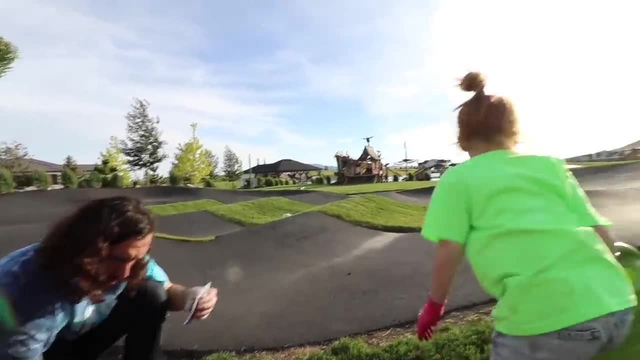 Good night, little flowers. See you when you grow up. This one's gonna be fun. That'll be way funnier. Wait, we got water. now We need water. You get waters and I'll clean up the garbage. I'll go get more water. 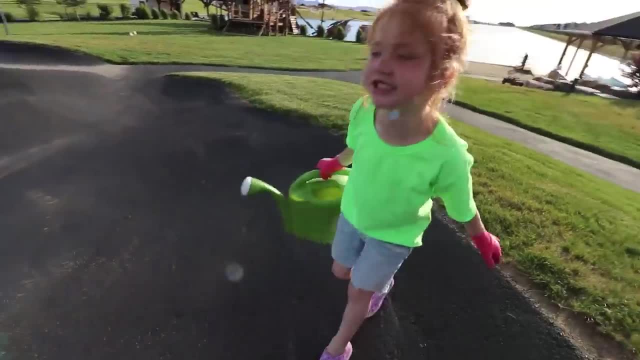 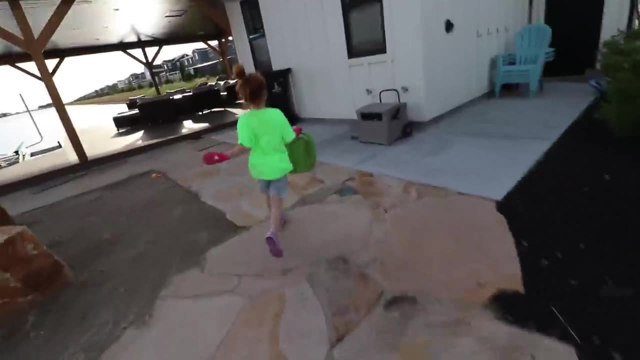 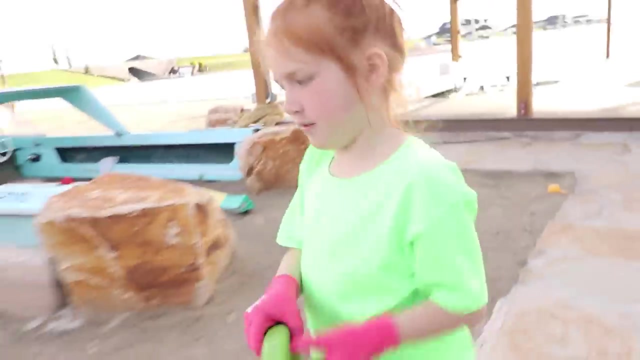 Can Dad waste it all on the dinosaurs? Hey, that's not wasting. They were thirsty, They weren't? You just made it up. Let's go get some water. Water, Okay, I think I'm all done. Let's go water right now. 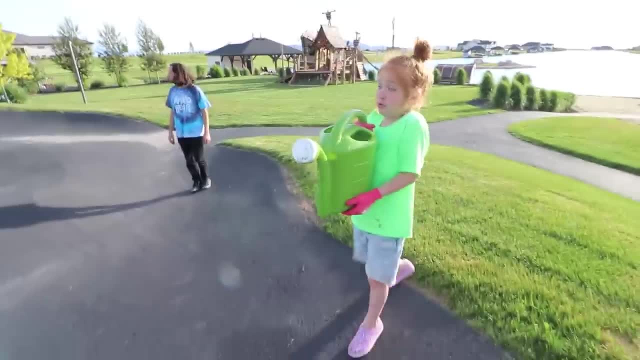 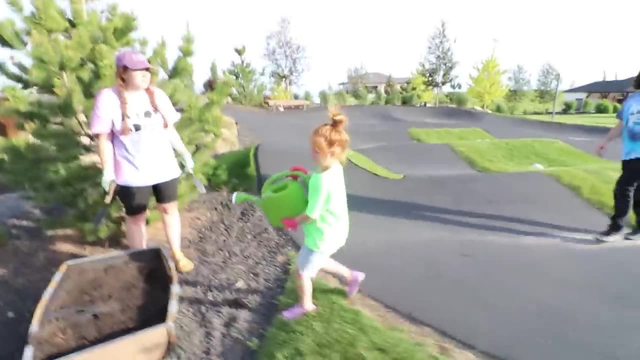 Wait, are we missing something? What? Where's Niko? I don't know, Mom, have you seen Niko? I thought he was with you. Niko, All right, let's water these babies, and then we gotta find a Niko's. 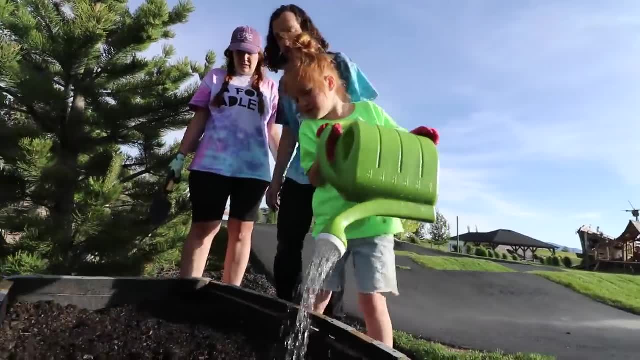 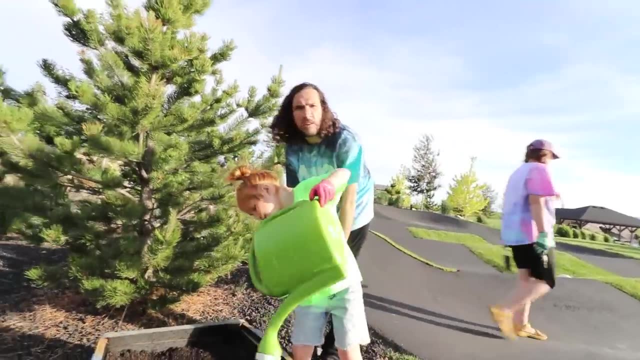 boy, This is how you water things: Da da da, da da da, Niko. have you seen, Niko? Okay, I think the cucumbers are gonna be extra healthy because this is extra wet. Okay, I think we need to find your brother. 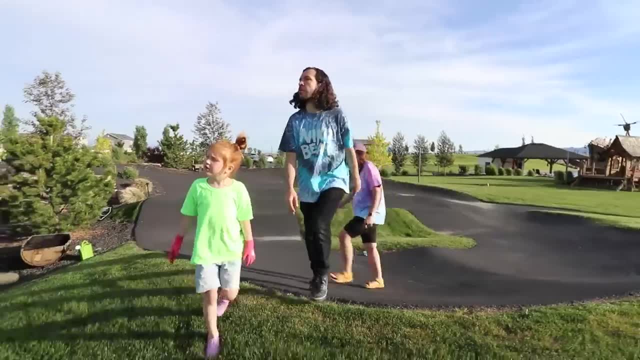 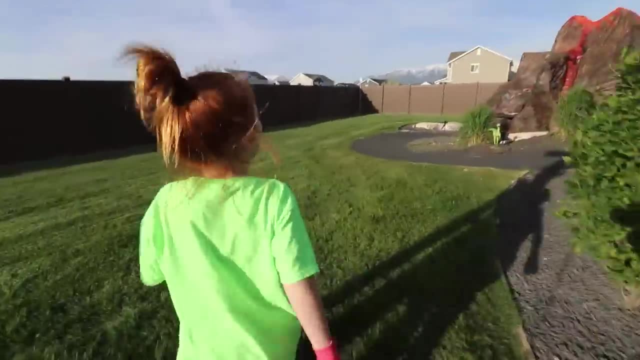 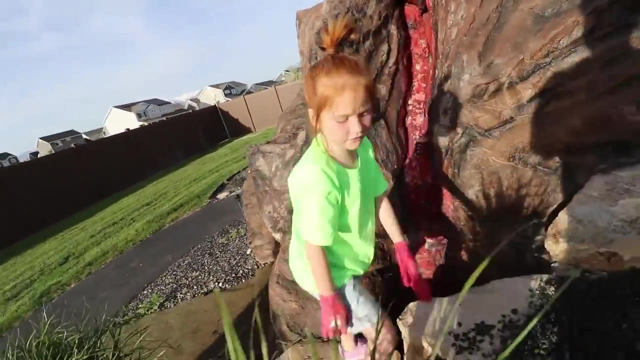 Wait, what if the volcano's open? Niko, we're gonna find you. Niko, Niko. This is his favorite spot. He's not there. That was his favorite hiding spot. Niko, Niko, Niko. 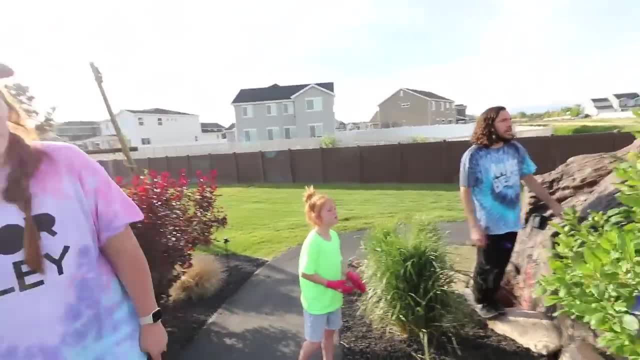 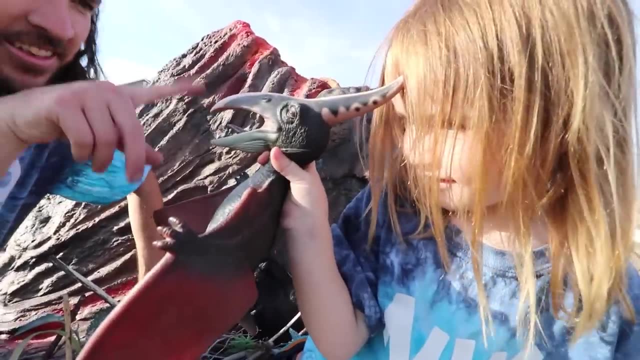 Niko, I see him. Or is that a pterodactyl? Is that a baby pterodactyl or a Niko? We found you. Are you in the pterodactyl nest? Hi little pterodactyl, Do you know where Niko is?